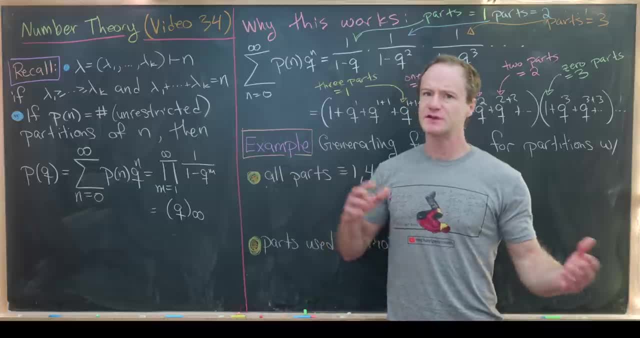 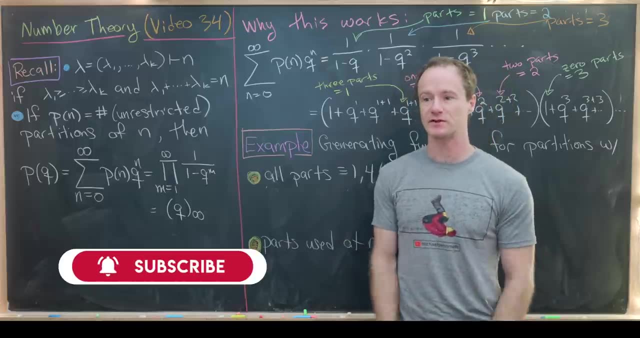 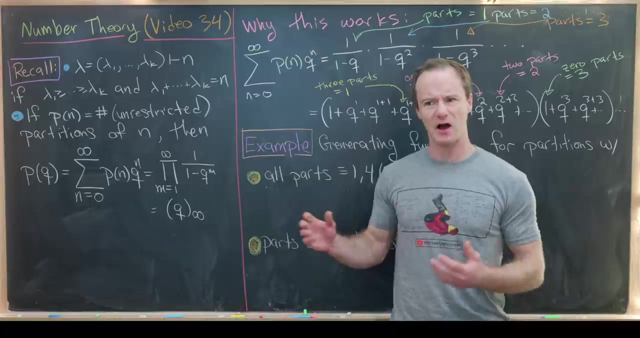 same Rogers-Ramanujan identity. Now, some of you guys might know that I started a series a long time ago with the aim of proving this identity, but I never got around to finishing it. Well, it turns out that I think this playlist is a better place to finish it, because I've covered. 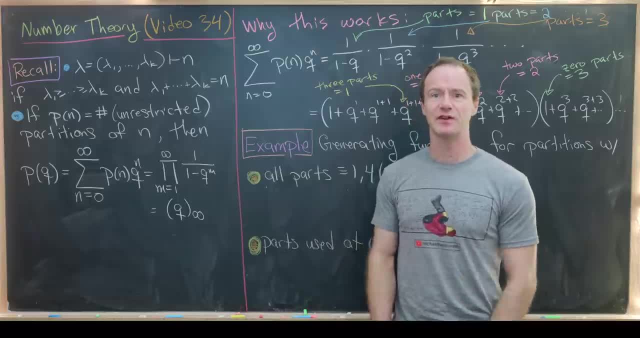 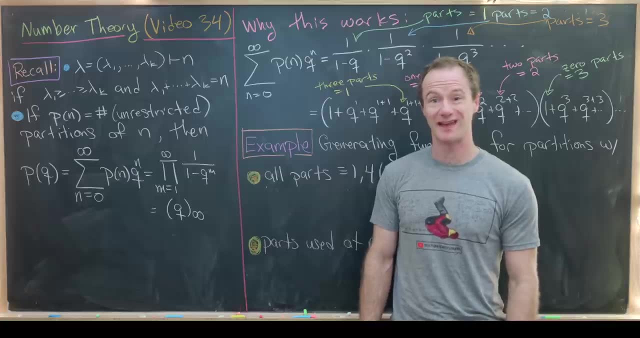 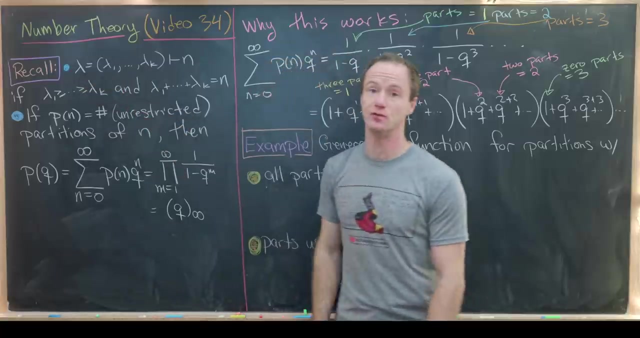 all of the necessary information And I think everything is done a little bit more nicely. Before we get into the major goal of this video, I want to recall a few things and look at some examples. So let's recall a partition of n named lambda is a k-tuple. This partition is said to: 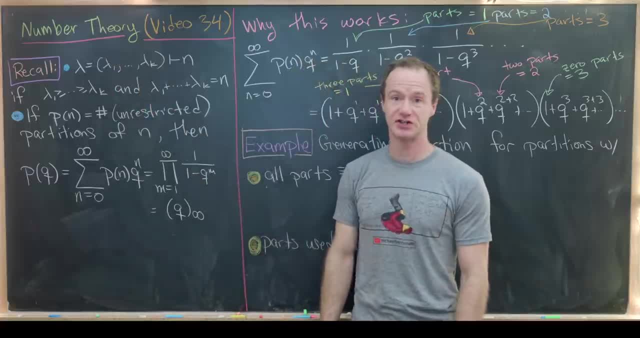 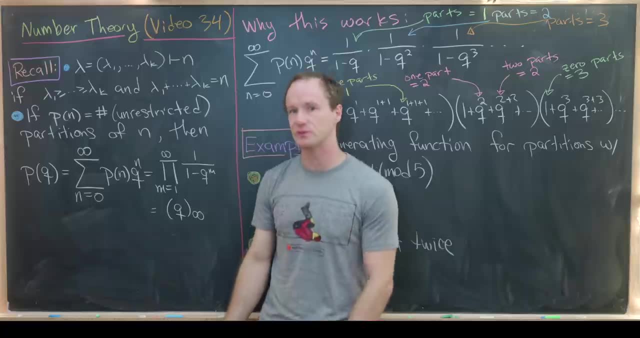 have k parts If it satisfies two of the following conditions: it is a k-tuple If it satisfies two conditions, so it's non-increasing. So, in other words, lambda 1 is bigger than or equal to lambda 2,, which is bigger than or equal to lambda 3, all the way down to lambda k, And I should really. 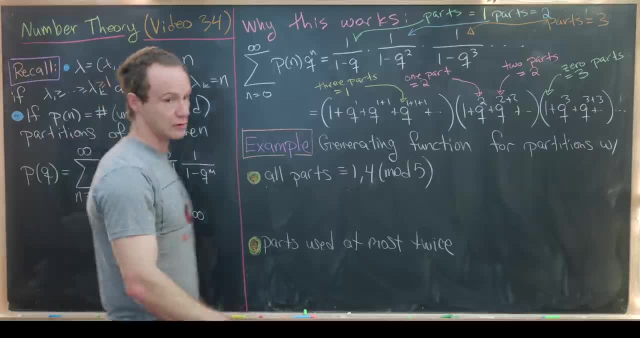 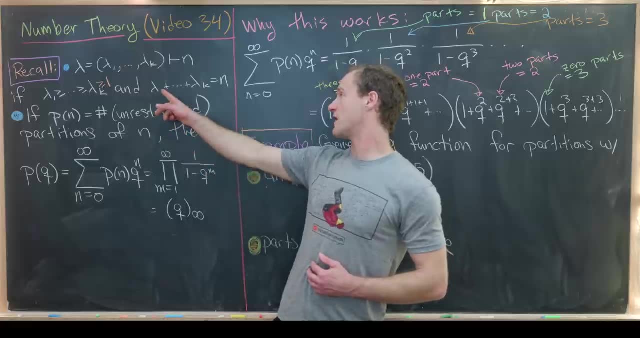 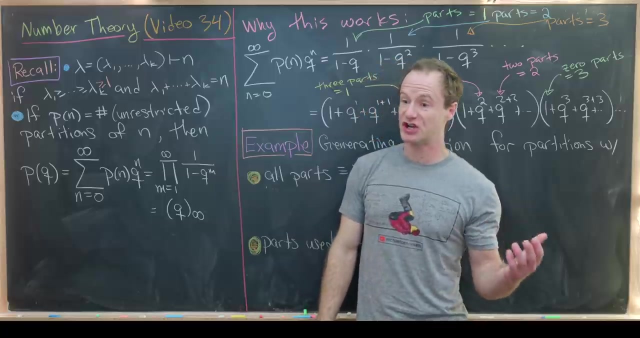 include here that lambda k is bigger than or equal to 1.. So these portions are made up of natural numbers, And then, furthermore, we have lambda 1 plus lambda 2, all the way up to lambda k is equal to n. Now let's recall that generating function is a k-tuple. So let's recall a partition of n named 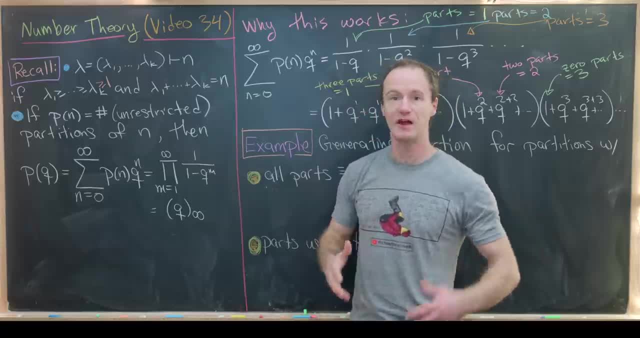 lambda k, And I think everything is done a little bit more nicely. Before we get into the major goal of this video, I want to recall a few more examples. So let's recall a few more examples. So, in other words, if we set a subsequence matrix of n and all the rest of the functions are an, 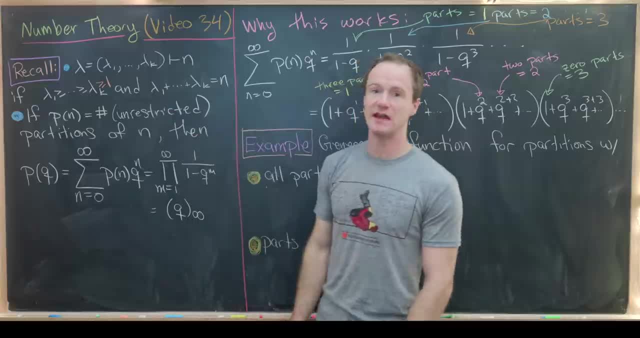 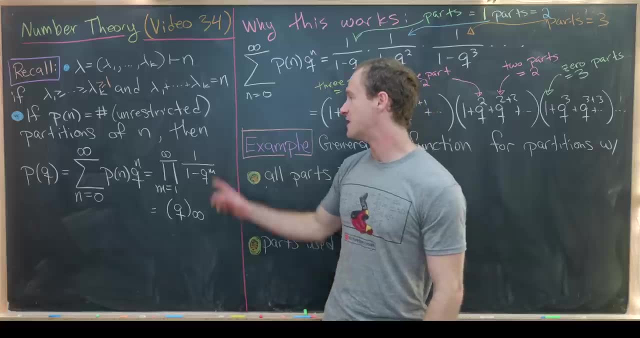 important tool for studying partitions and coming up with partition identities, as we've seen in previous videos. So if we set P of n equal to the number of unrestricted partitions of n- that's sometimes called the partition function- Then the generating function for P of n, sometimes called 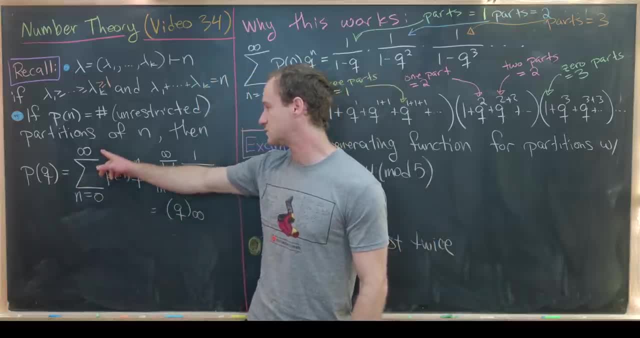 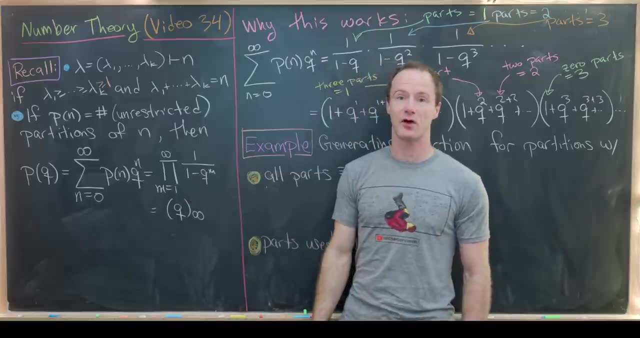 P of q. So that's going to be the sum, as n goes from 0 to infinity, of P, of n, q to the n, Where we take P of 0 to be 1.. that's equal to this infinite product of things that look like sums of geometric series. 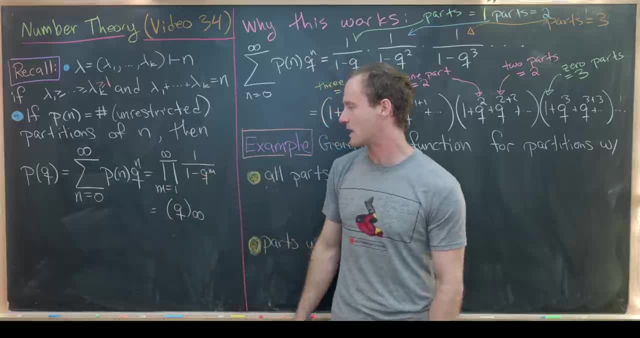 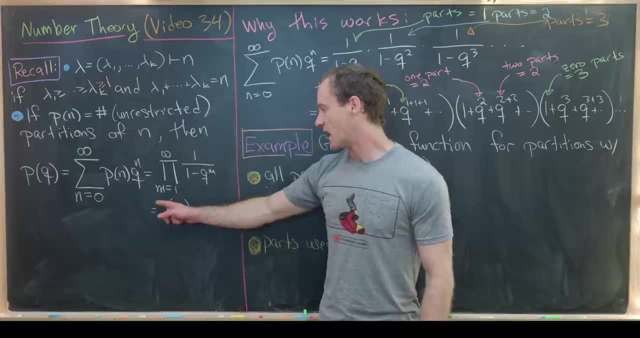 So the product is: m goes from 1 up to infinity of 1 over 1 minus q to the m, And we had some notation in previous videos using this thing called the Pockhammer symbol that allowed us to write this as this: q in parentheses with an infinity. 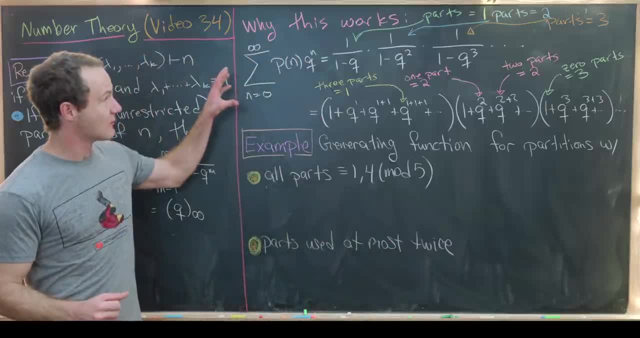 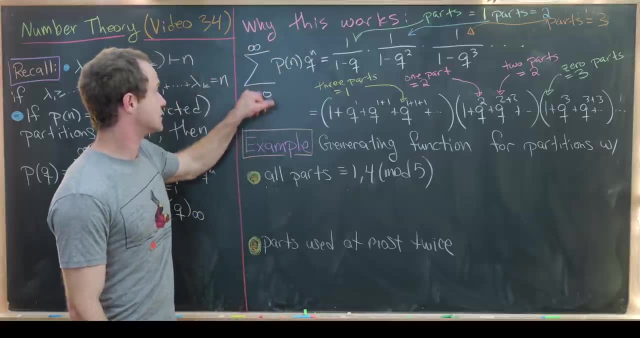 Now, before we get into the main goal of the video, I want to recall why this generating function works. So if we take this sum as n goes from 0 to infinity of p, of n, q to the n, and write it out as the product, 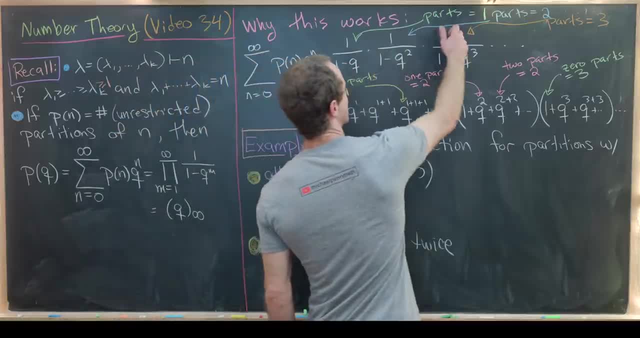 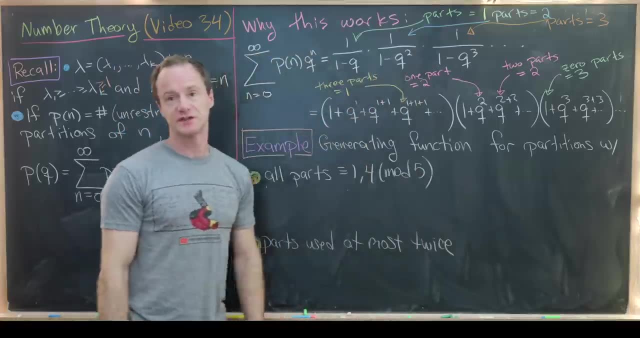 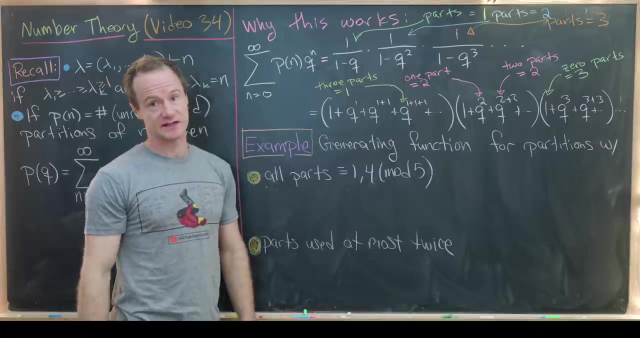 So we've got 1 over 1 minus q, 1 over 1 minus q squared, 1 over 1 minus q, cubed, and so on and so forth forever. Then each of these portions of our rational function or our infinite product give us certain things related to the partitions. 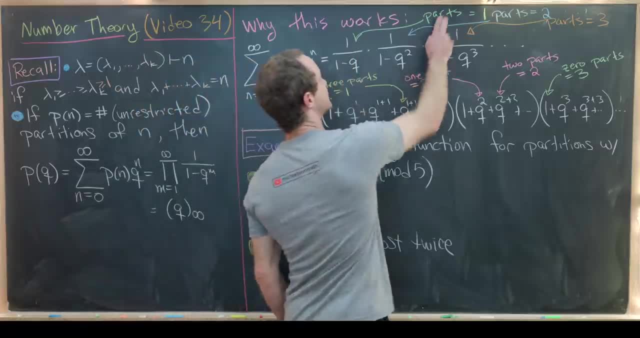 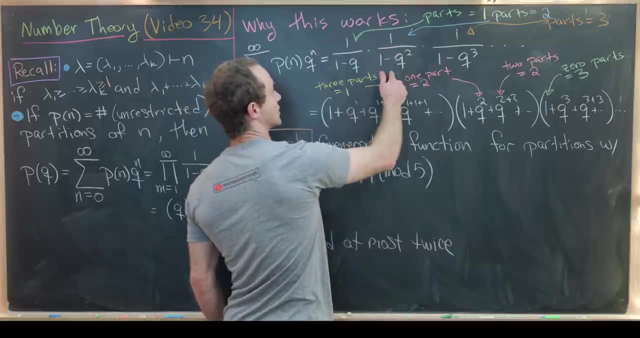 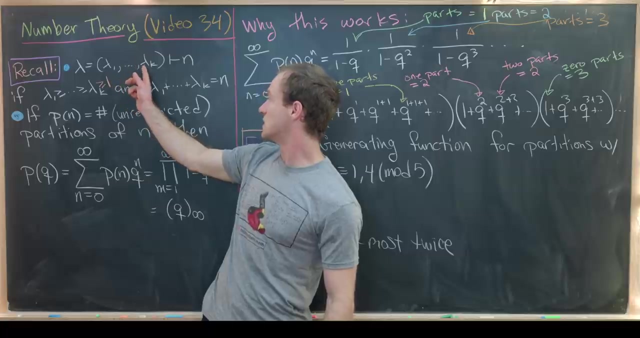 So this 1 over 1 minus q controls The parts of each partition that are equal to 1.. This 1 over 1 minus q squared term controls parts of the partition that are equal to 2.. And what I mean by parts, that's these individual things that are making up the partition. 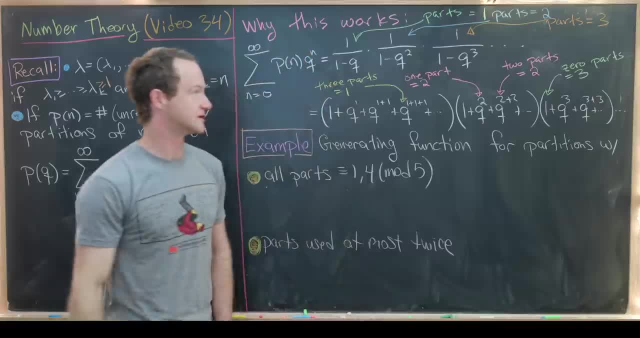 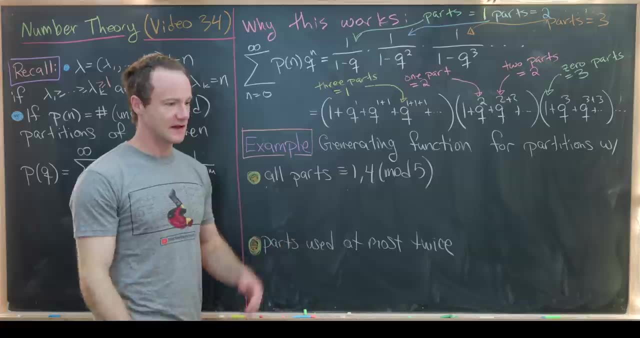 And then 1 over 1 minus q. cubed, those are parts that are equal to 3.. Furthermore, if we expand each of these as geometric series- which you should really think about these as being expanded as geometric series. that's the more proper way to view this infinite product. 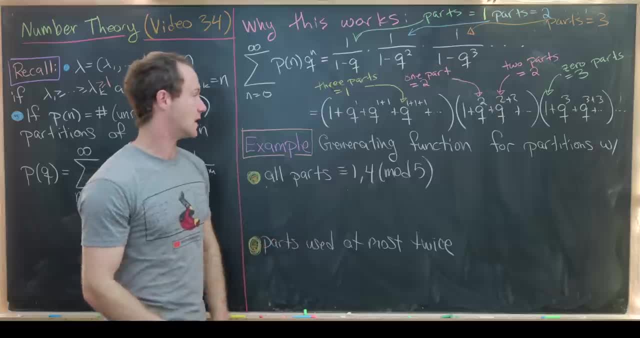 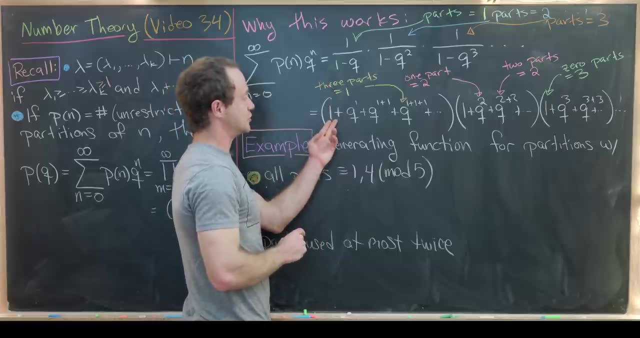 We can see a little bit more of what's going on. So, for instance, this 1 over 1 minus q, we can think of it as expanding to 1 plus q, to the first q, to the 1 plus 1, q to the 1 plus 1 plus 1.. 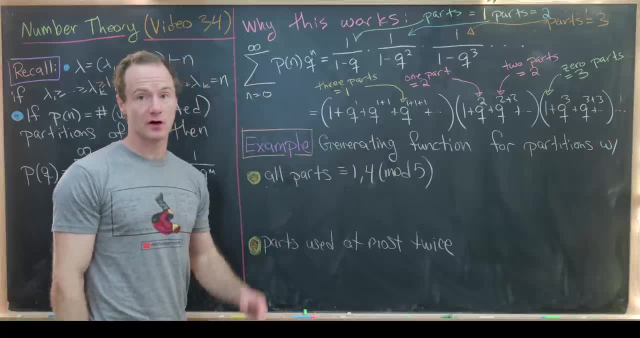 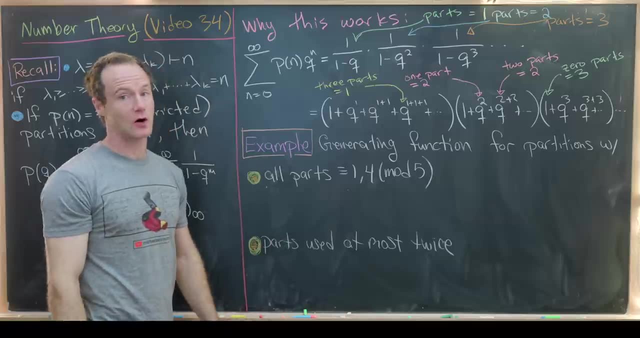 And each of these controls how many parts of the partition are equal to 1.. So this number 1 here corresponds to not using the partitions, Not using 1 at all in the partition. This corresponds to a single part which is equal to 1.. 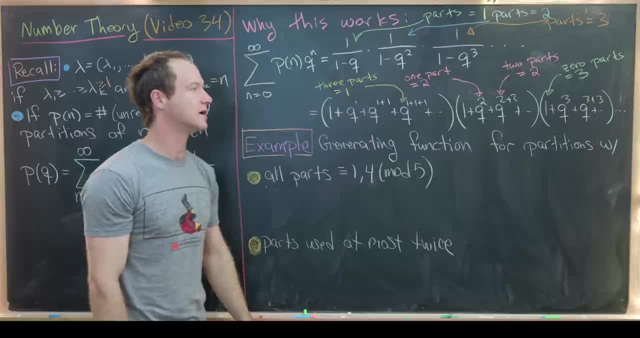 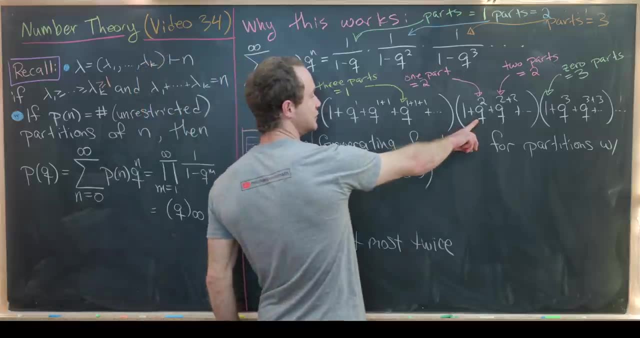 Here we have 2 parts equal to 1,, 3 parts equal to 1.. And then we've got similar rules for 2,, 3,, 4,, 5, 6, and so on and so forth. So this q squared corresponds to 1 portion of the partition equal to 2.. 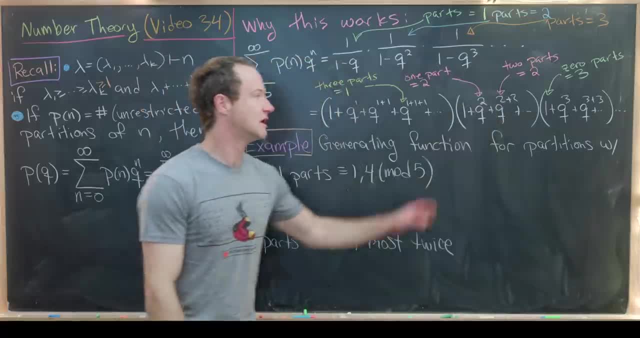 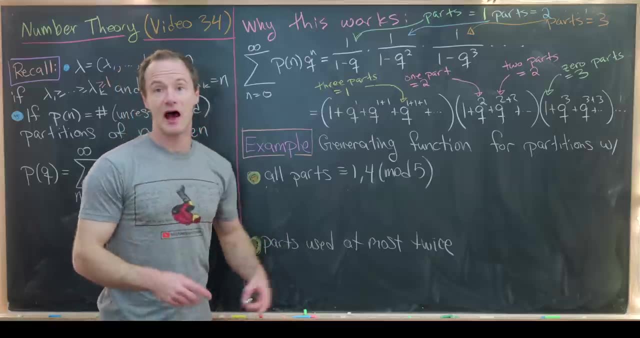 This q to the 2 plus 2 is 2 parts equal to 2.. And then, well, that continues on. So let's look at some examples real quick, Just to recall, maybe, how these things are built. Let's find the generating function for partitions, where all of the parts are. 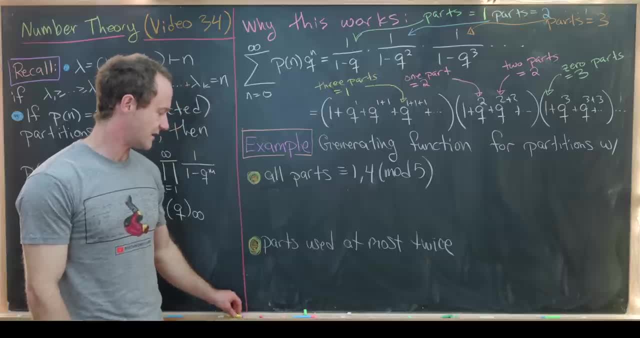 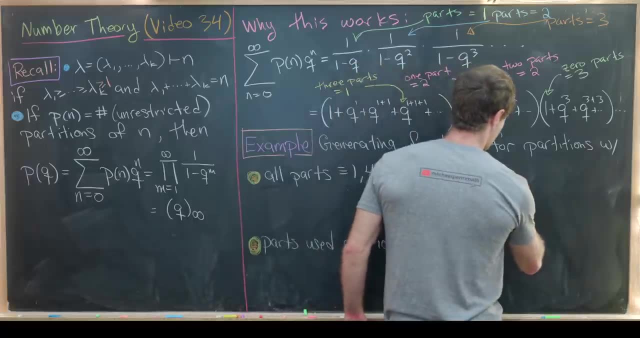 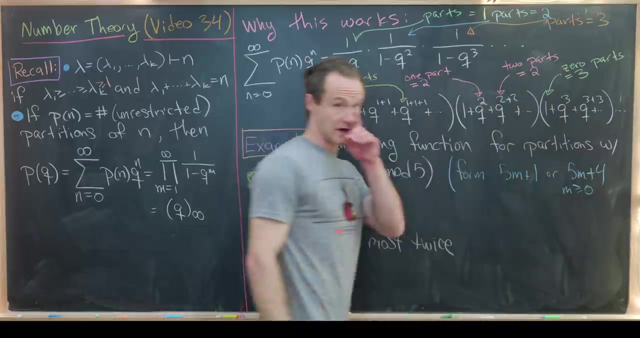 congruent to 1 or 4 mod 5.. Let's first recall that being congruent to 1 or 4 mod 5 means that we are of the form 5m plus 1 or 5m plus 4, where m is bigger than or equal to 0.. 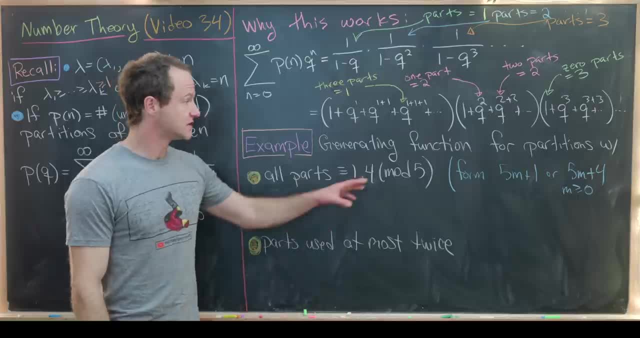 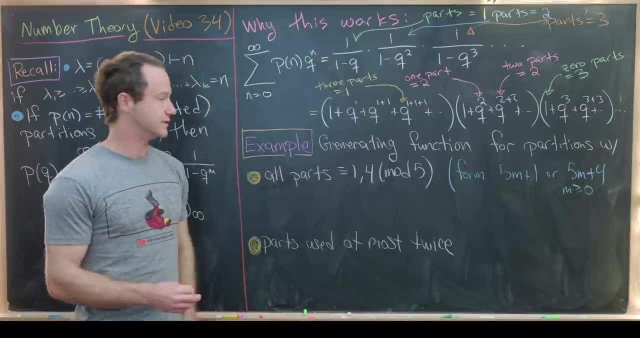 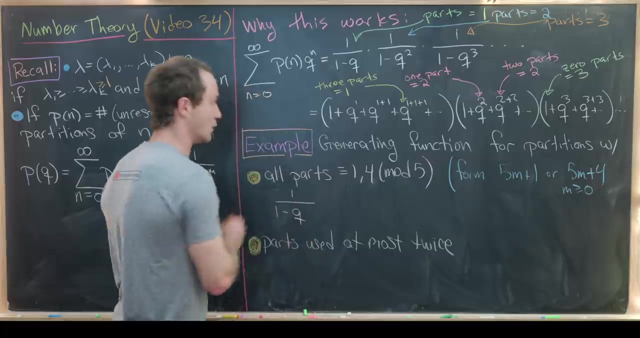 But m could be anything bigger than or equal to 0.. So, keeping in mind that these types of rational functions control what parts we're using, we can write down a generating function pretty easily and it would look like this: 1 over 1 minus q to the 1 power. 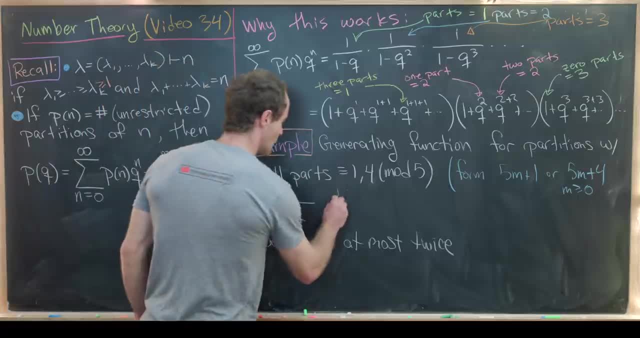 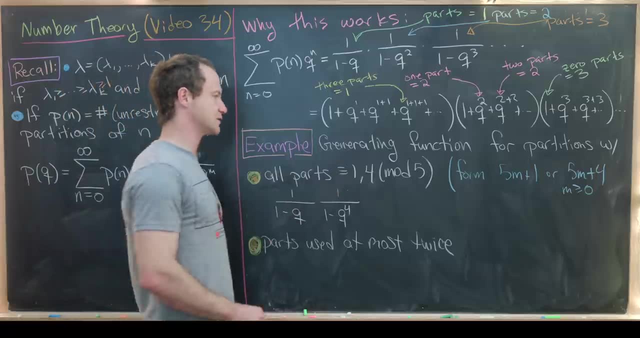 That would be using a part that is equal to 1.. 1 over 1 minus q to the 4th power, That would be parts equal to 4.. And then the next number, that is 1 mod 5, is 6.. 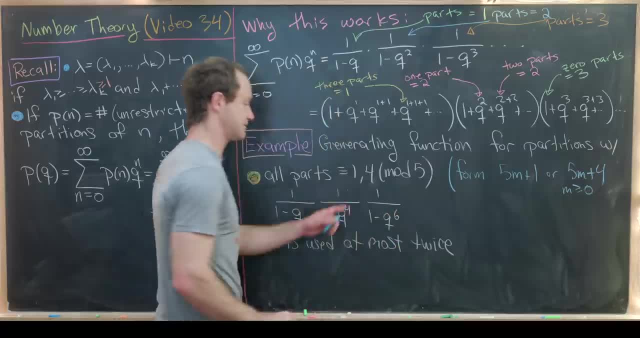 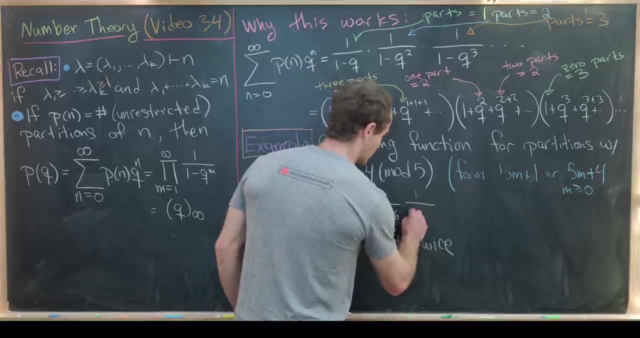 So that's what we would have next: 1 over 1 minus q to the 6.. Those are using parts that are 6.. The next number would be 9, because that is 4 mod 5. So 1 over 1 minus q to the 9.. 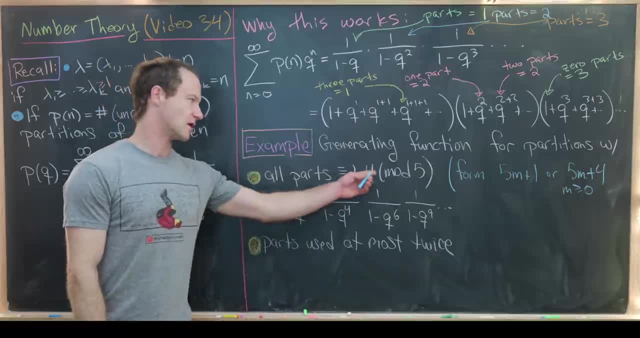 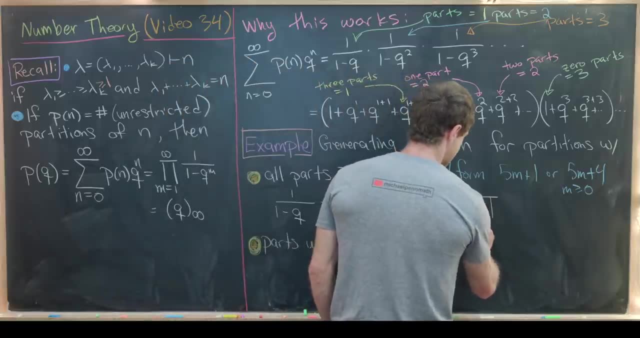 And that's going to end up being an infinite product, because there are infinitely many numbers that are congruent to 1 or 4 mod 5.. We could end up writing this as the product as m goes from 0 up to infinity of 1 over. 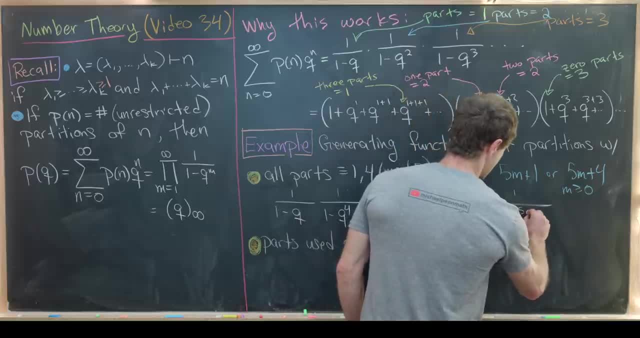 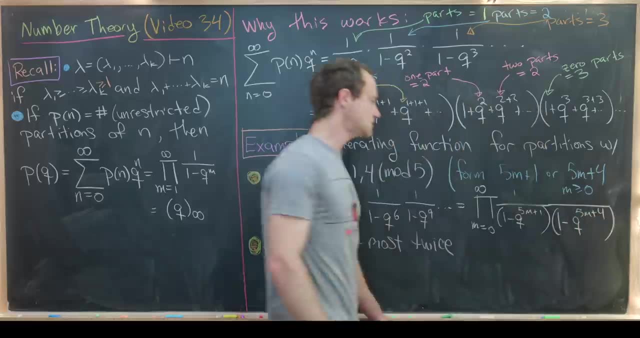 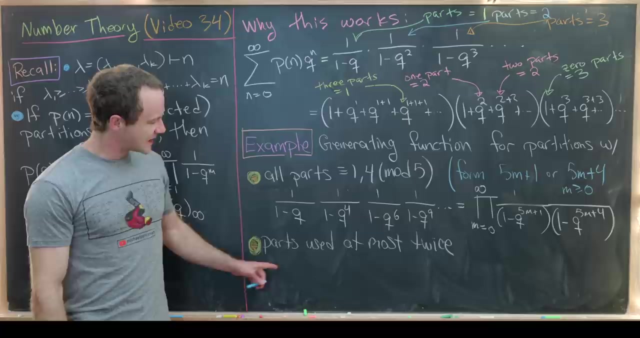 1 minus q to the 5m plus 1.. And there's a simplified way to write that down using our pockhammer symbol, which I'll have come on the screen right now. Now we could do something else. Let's say we wanted to find the generating function for partitions where the parts are. 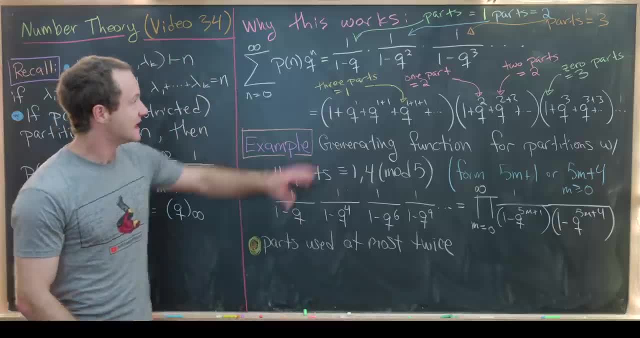 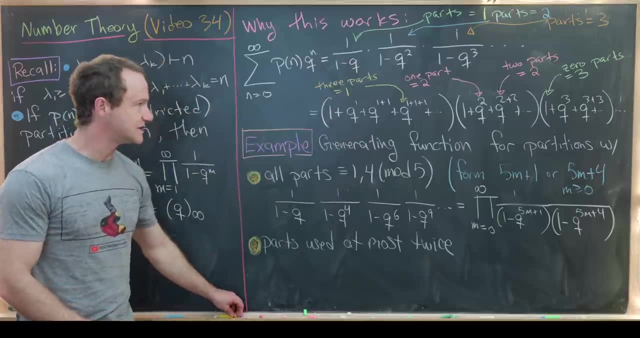 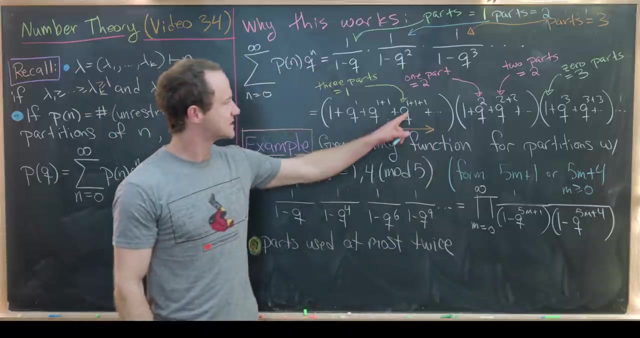 used at most twice. Then instead of thinking about the rational function, we want to think about its expanded form. So only using them twice. Twice means that we cannot include anything past this point, because this q to the 1 plus 1 plus 1 corresponds to using the number 1 three times. 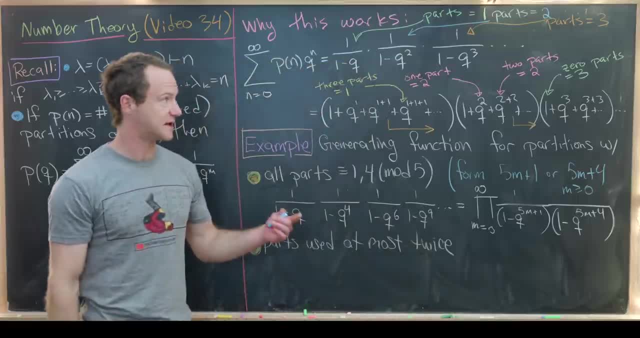 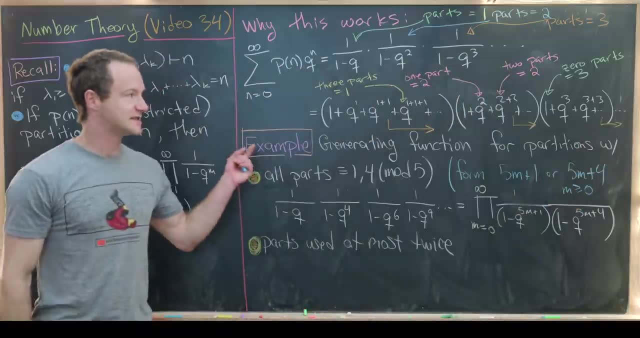 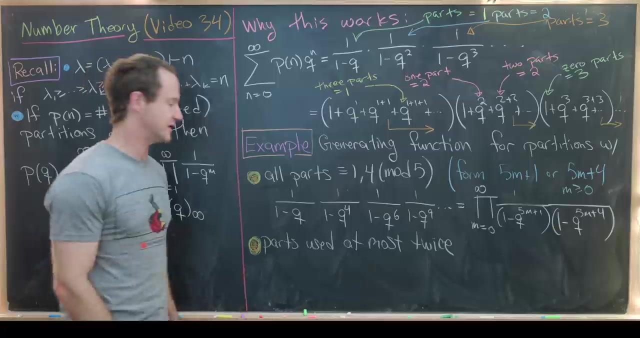 And then, furthermore, everything past this point corresponds to using the number 2 three or more times, and then so on and so forth, like this. So that means, instead of an infinite product of geometric series, we have an infinite product of just polynomials. 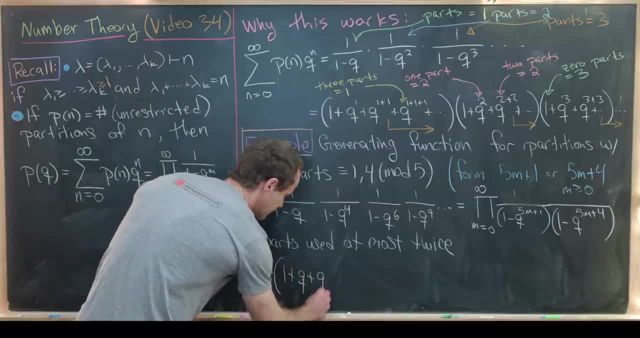 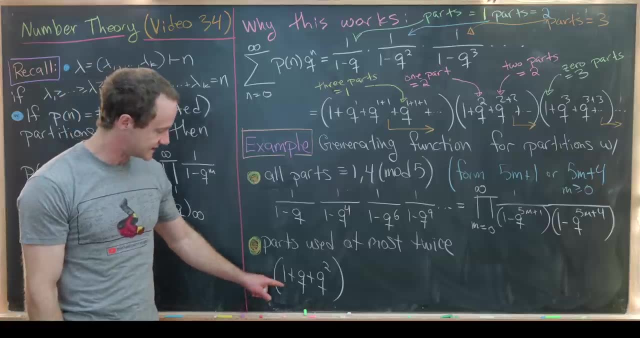 So here we'll have 1 plus q plus q squared. I'll write it as q squared instead of q to the 1 plus 1.. So that corresponds to using 1,, 0,, 1, or 2 times, And then we'll have 1 plus q squared plus q to the 4th. 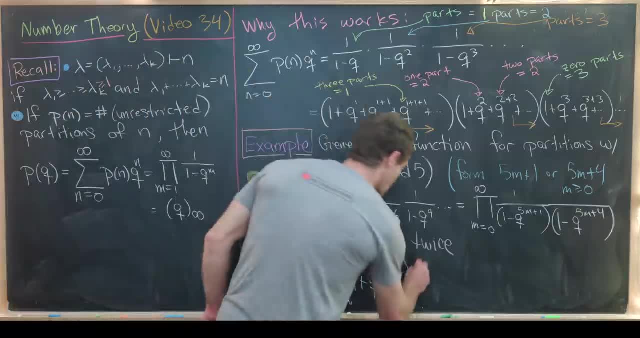 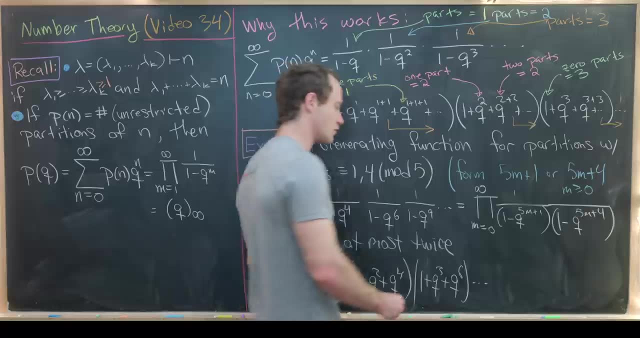 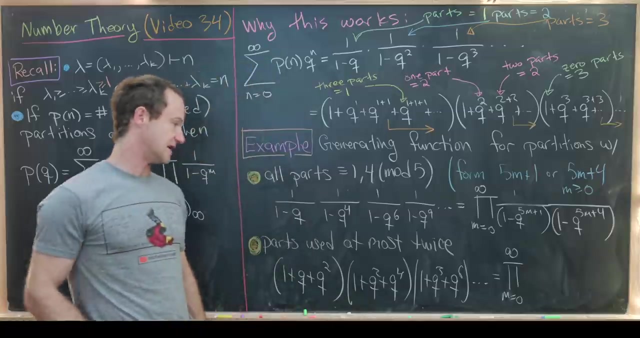 That corresponds to using 2, 0, 1, or 2 times 1 plus q, cubed plus q to the 6, and then so on and so forth. Okay, We could write that with a product notation As the product as m goes from 0 up to infinity of, or maybe we should go from 1 up to infinity. 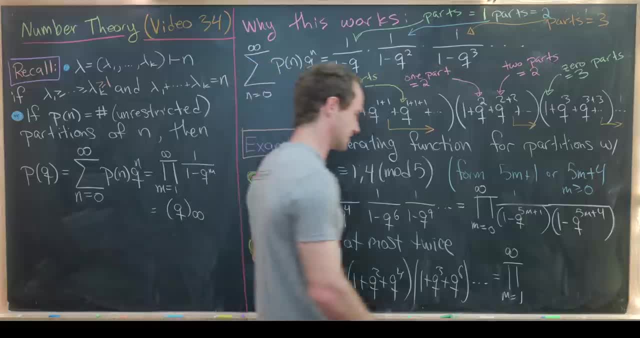 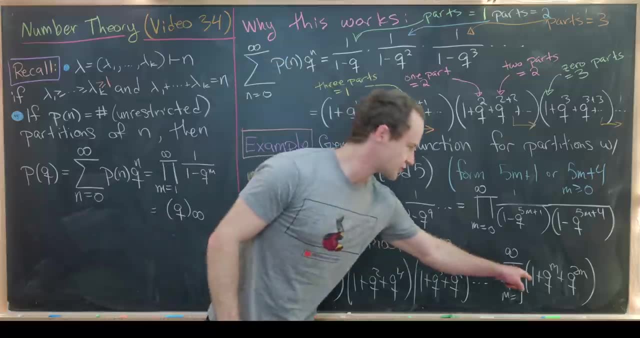 in this case I think it'll be written down a little bit nicer. Then we'll have 1 plus q to the m plus q to the 2m. So this portion would be like, using a part which is equal to m, 0 times 1 time, or 2. 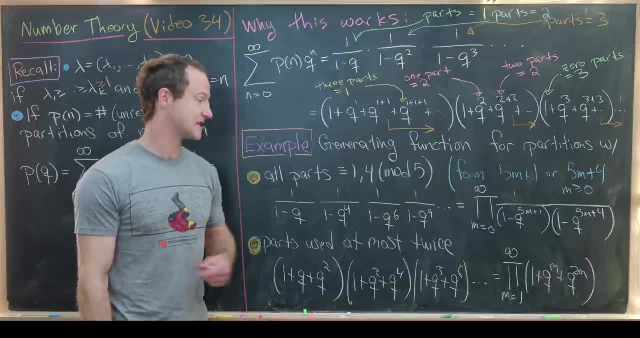 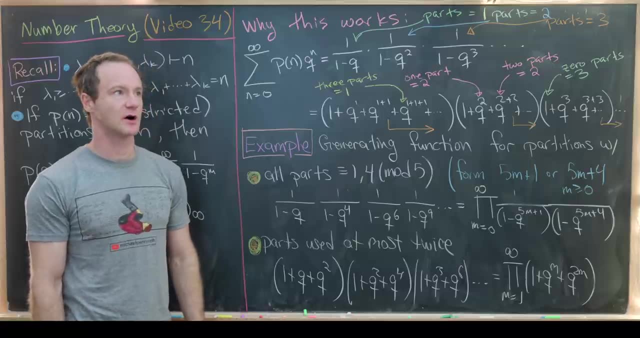 times. Now there's a nice identity that I assigned to my class which allows us to write this object In another form, which represents partitions, where the parts are congruent to 1 or 2 mod 3.. That's so. that's a pretty famous result. 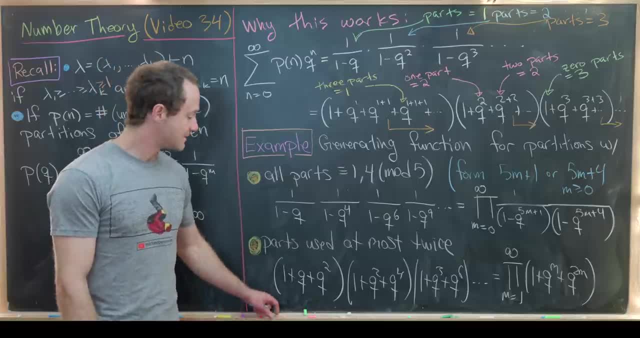 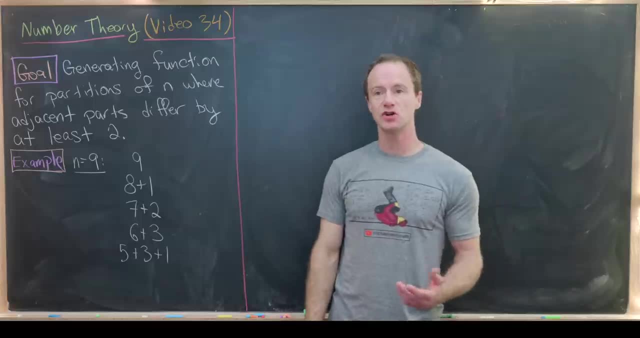 I'll let you guys try that on your own if you're interested. Okay, So now that we've got this kind of review under control, let's see what our main goal for the video is. So our major goal for this video will be to find a generating function for a certain type. 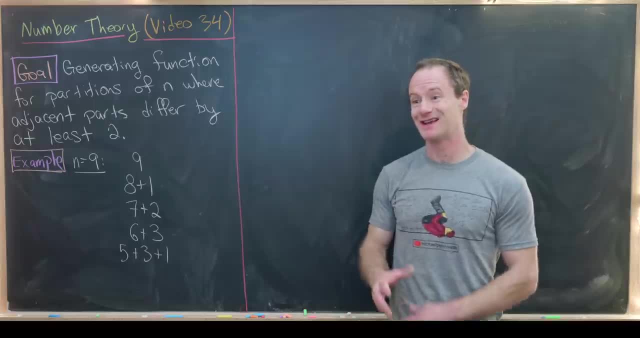 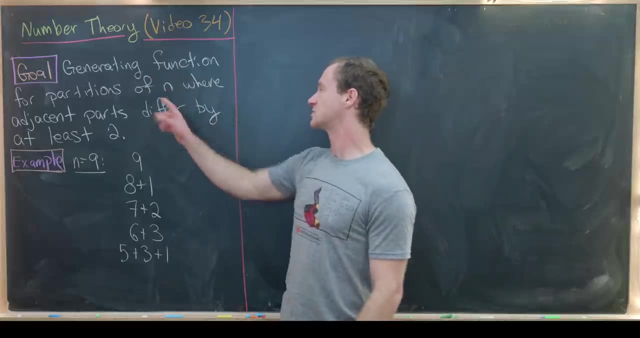 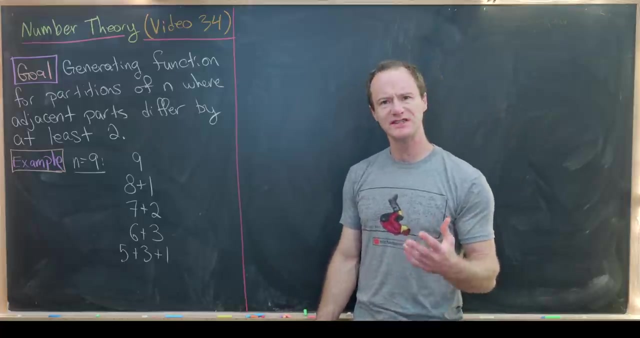 of restricted partition. But that restricted partition is not quite as simple As the ones that we just looked at. In particular, we want to find the generating function for partitions of n where adjacent parts differ by at least 2. So just as an example, although you could easily write down a lot of other examples- 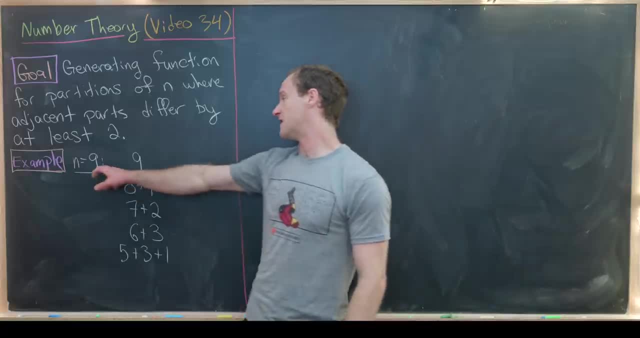 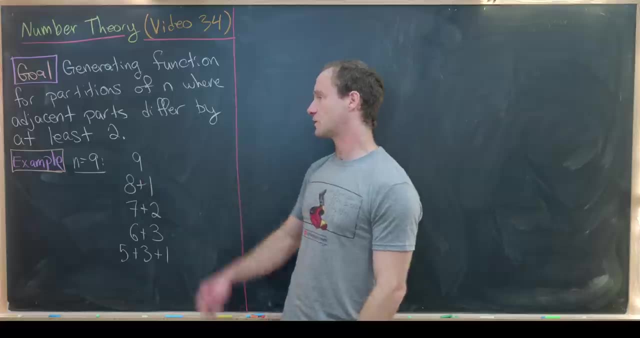 and I urge you to, to get a feel for what these look like. If n equals 9,, we have 5 total partitions that satisfy this rule, So the first one will be 9.. Well, that has a 7.. That has a single part. 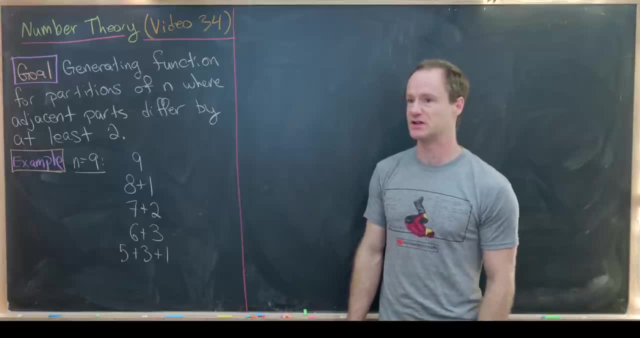 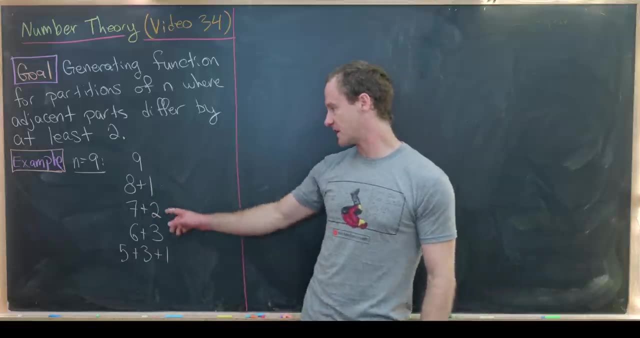 But that means there's no adjacent part to have this difference condition. So we're good to go there. So the next one is 8 plus 1.. 8 and 1 clearly differ by at least 2.. 7 plus 2, 6 plus 3 are the other ones that have length 2.. 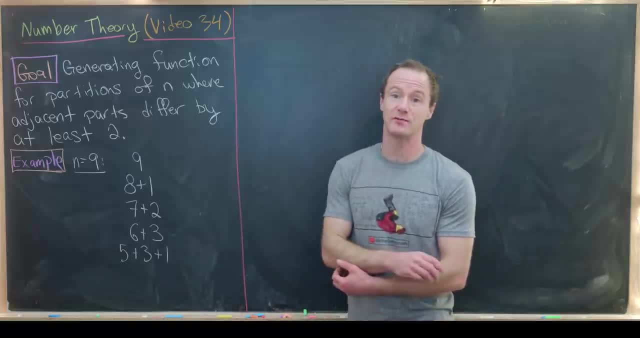 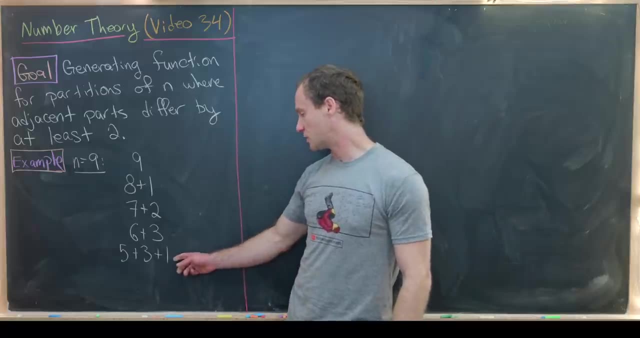 So notice. the next one, kind of in this vein, would be 5 plus 4.. But the difference between 5 and 4 is not at least 2. So we go down to a partition of length 2. And that would be 5 plus 3 plus 1.. 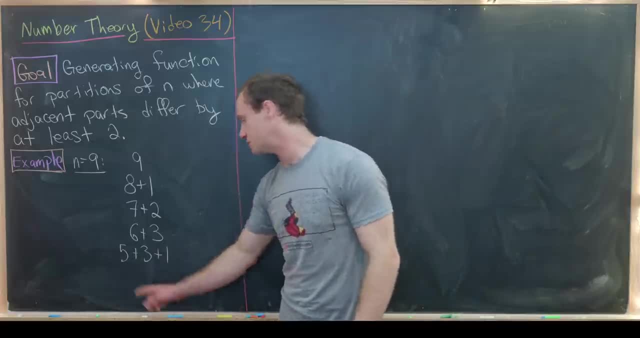 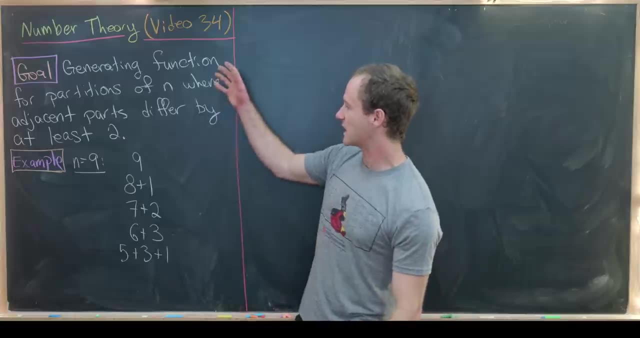 So notice that sums to 9.. And there's a difference of 2 between each one, And this represents all such partitions that satisfy this rule. OK, so now that we've got an idea of the goal, I need to define a couple of functions, which. 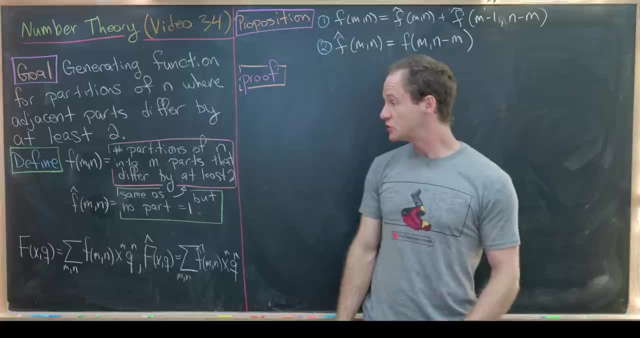 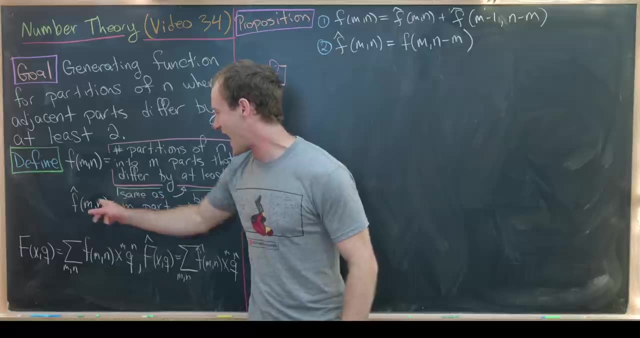 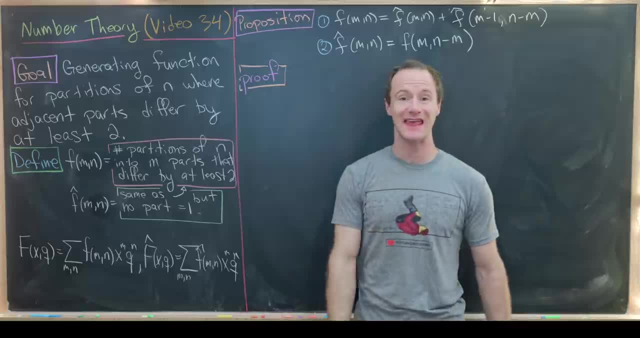 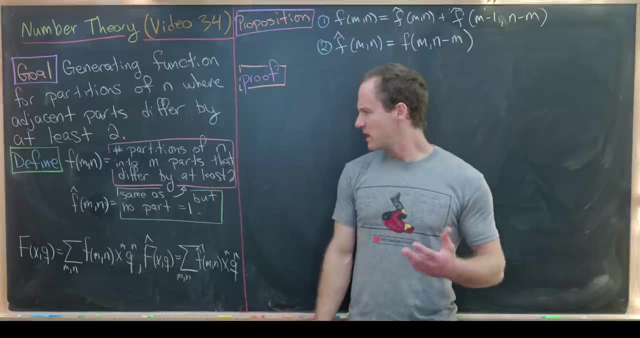 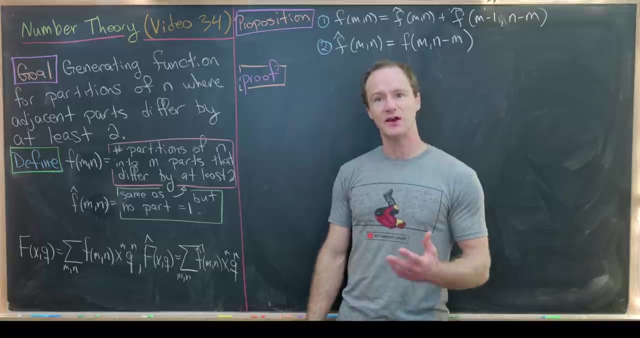 So f of mn is the number of partitions of n into m, parts that differ by at least 2.. So maybe, if you're having trouble figuring out what this means, look back at our example, for n equals 9. And notice that m could be equal to 1,, 2, or 3 in that case. 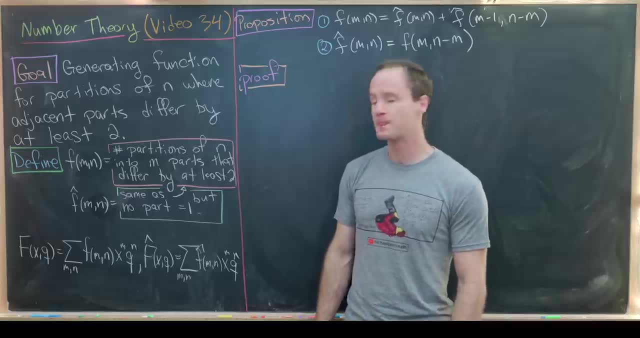 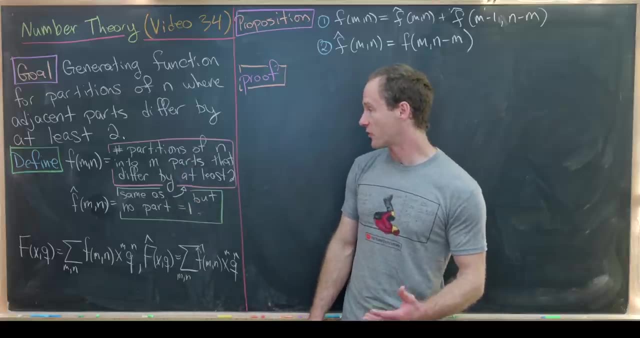 If m was bigger than 3, then we would get 0 for this. OK, and then f hat of mn has the same number of parts. It's the same condition as this one up here, In other words, it's partitions of n into m, parts that differ by at least 2.. 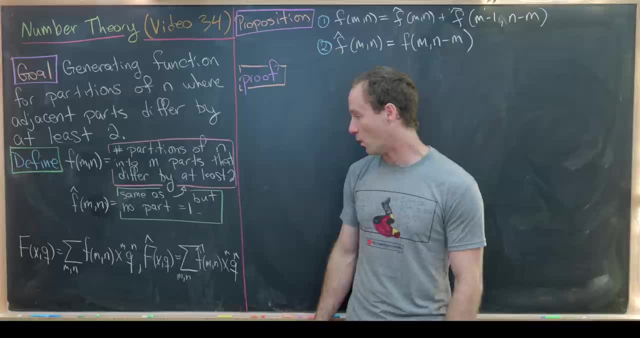 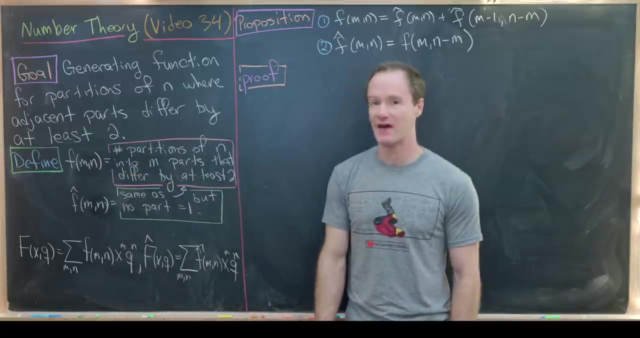 But in this case none of the parts are equal to 1.. So that means the smallest possible part here is equal to 2.. And then, since we're looking for generating functions, I will define two 2-variable generating functions, based off of f and f hat. 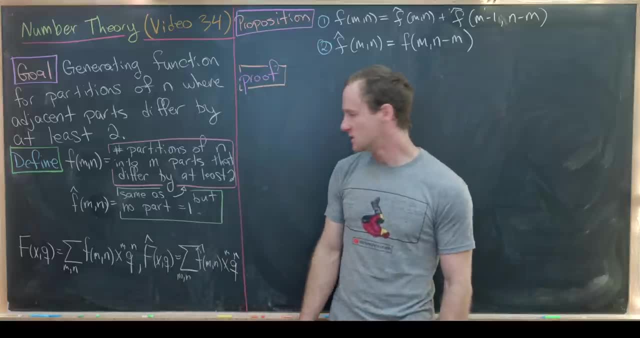 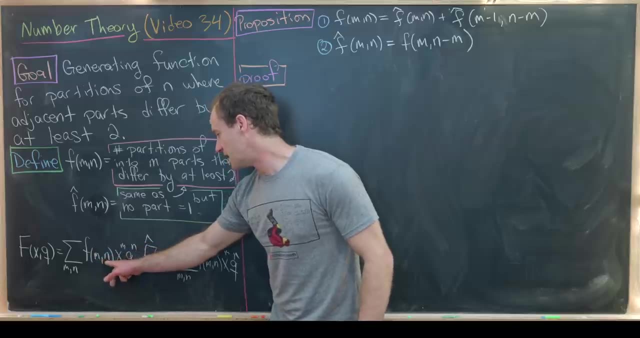 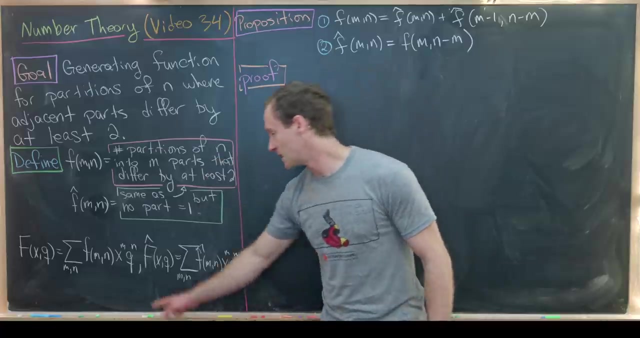 So I've called them capital F and capital F hat. So capital F of xq is the sum over m and n. So it's a double sum, F evaluated at mn, x to the m, q to the n. So our x variable is counting the number of parts. 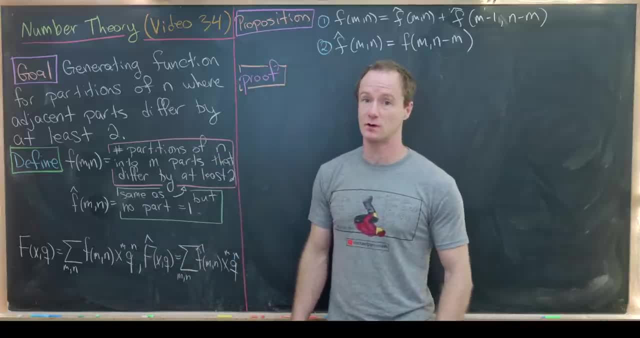 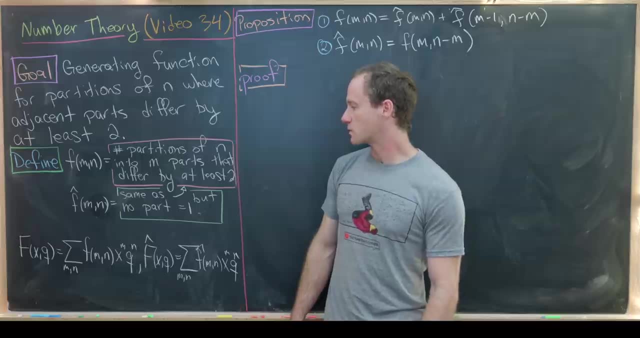 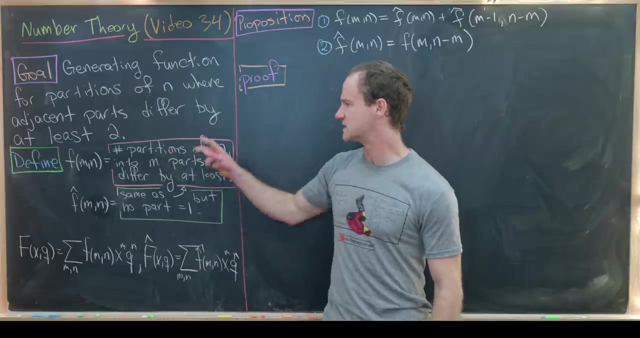 And our n variable is counting the partition that we're looking at, And then f hat of xq is defined similarly, just with f hat here. So remember, our goal is to find the generating functions for parts like this, And so that would be related to this pink box here. So we'll start with the following. 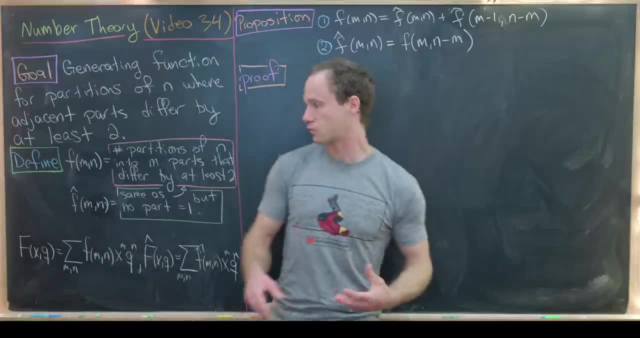 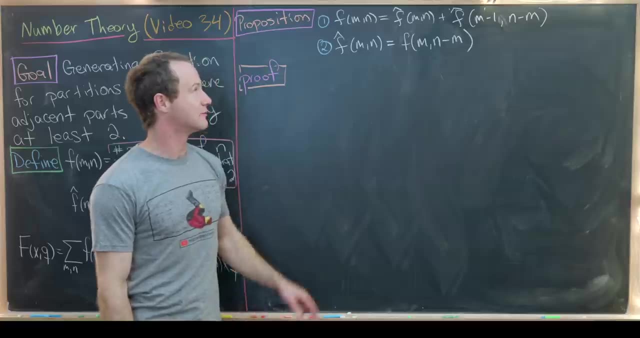 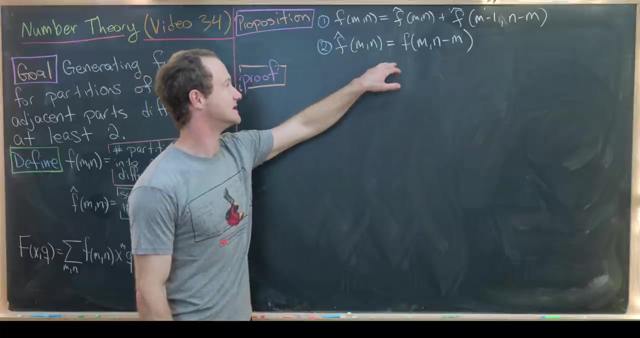 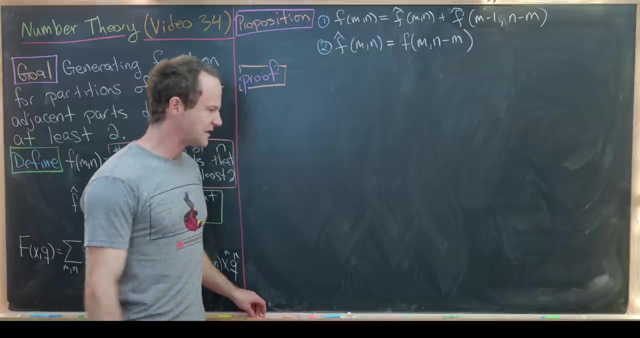 proposition. It has two parts and it's some sort of recursion between these two functions. So we've got: f of mn is equal to f hat mn plus f hat m minus one, n minus m. And then the second one is: f hat mn is equal to f mn, n minus m. Okay, so let's see how this proof goes, And I think 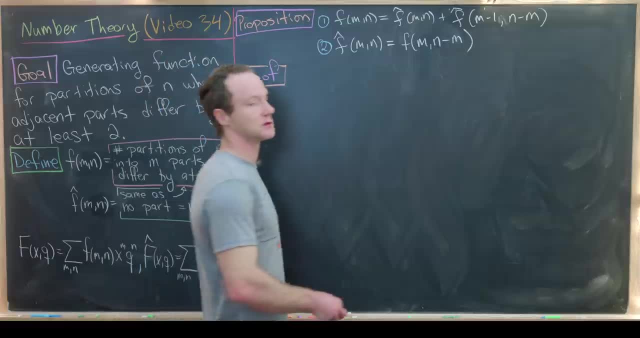 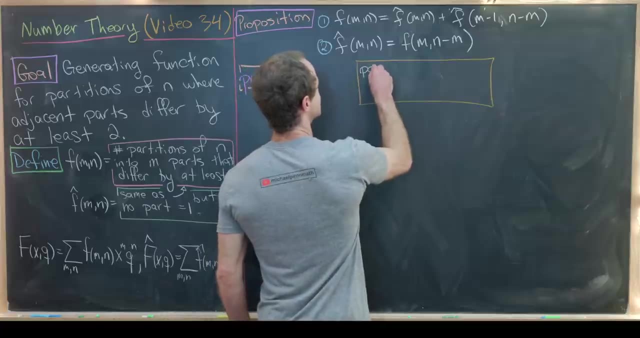 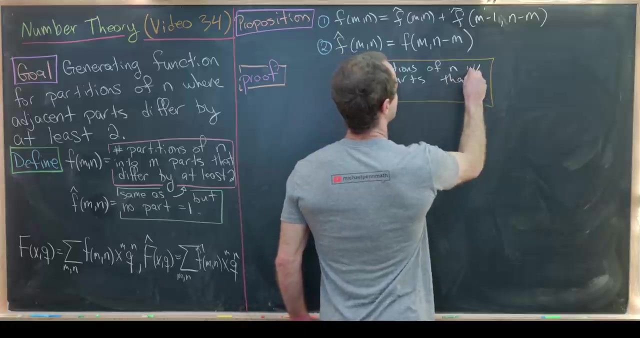 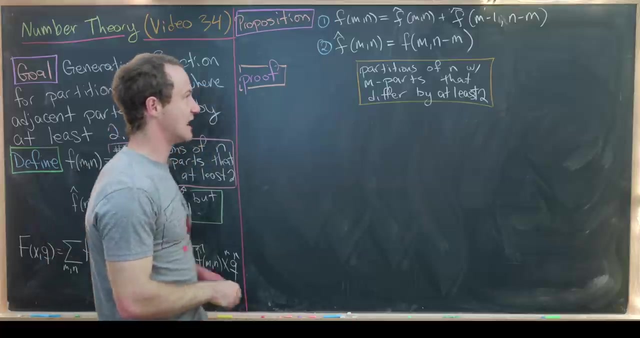 maybe the best approach to this proof is like kind of visual. So let's start up here and say that this box contains all partitions of n with m, parts that differ by at least two. So by the definition of our function over here, we know exactly how many elements are. 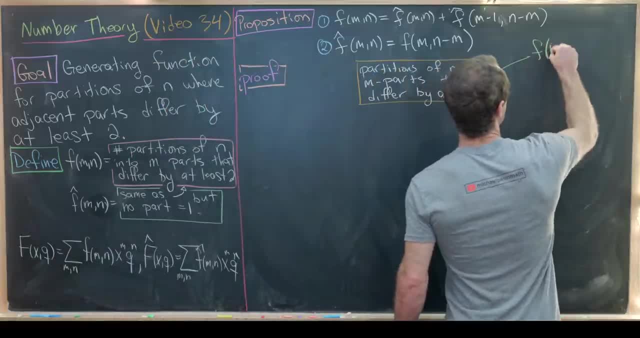 in there. So we know exactly how many elements are in there. So let's start up here and say that. So by the definition of our function over here, we know exactly how many elements are in there, this box, So there are f m n elements in this box. by the definition of f m n And then looking up, 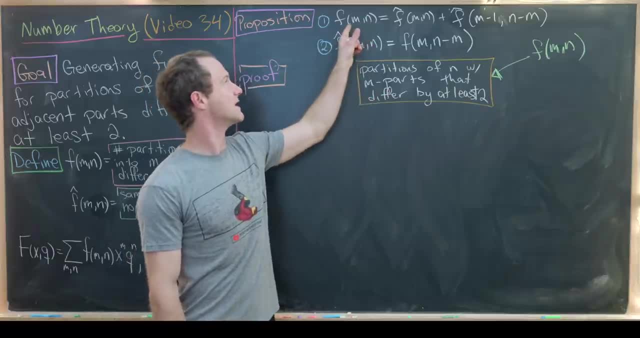 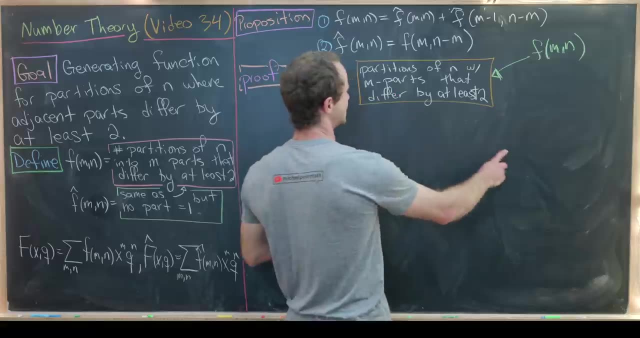 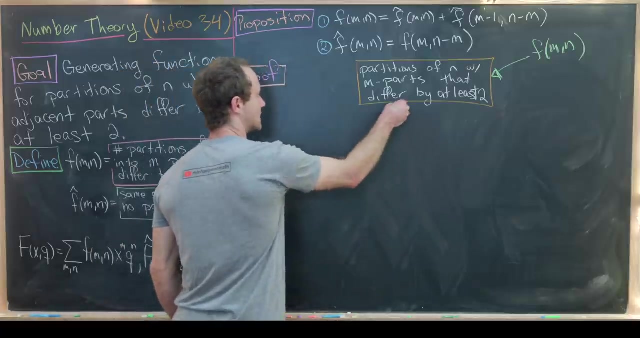 at our goal. we see that we want to separate this number, f m n, into two pieces. So that means we should probably take each of the elements in this box and naturally partition them into two, maybe like sub boxes we could call it. So I'll bring one down here to the left and one down here to the 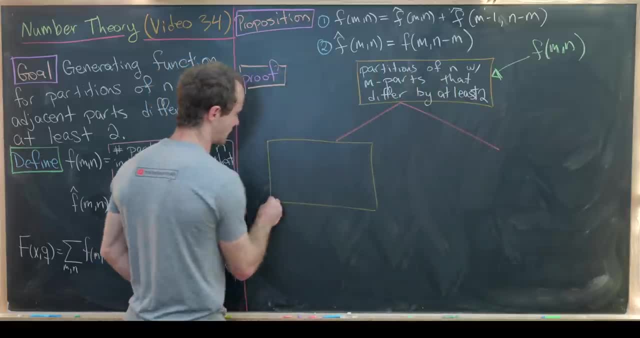 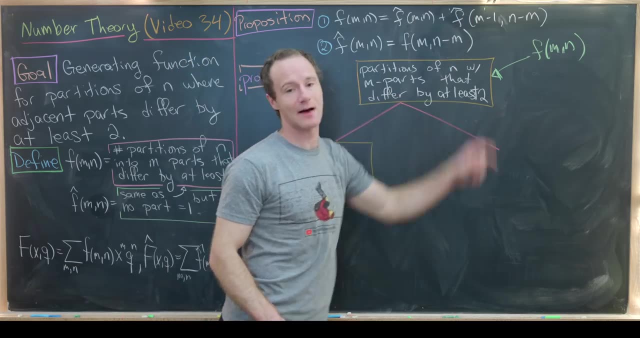 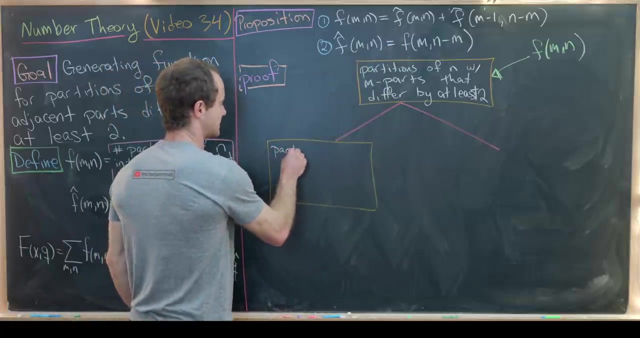 right, Let's see. how should we do this? Well, obviously, we should do this in a way so that one of them contains f, hat, m? n elements and the other one contains that many elements. Well, it turns out it's easy to do this one. So notice that these will be partitions of n, with m parts differing. 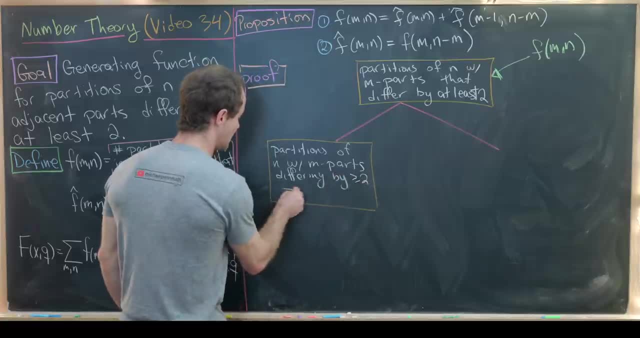 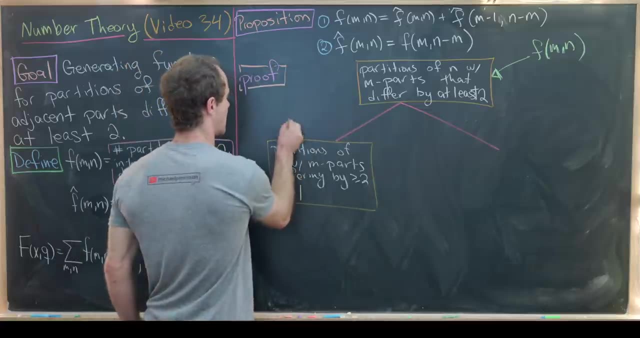 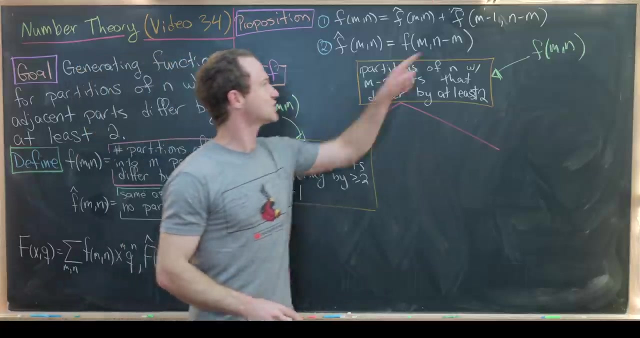 by b Bigger than or equal to two, and then here not equal to one. That's like the definition of this f hat m? n. So that means there are f hat m? n elements in this box. Okay, so we can't just write. 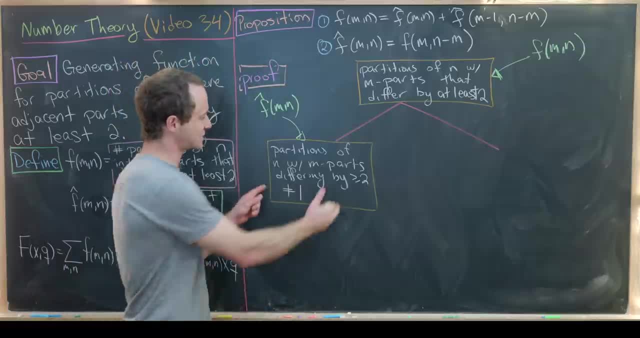 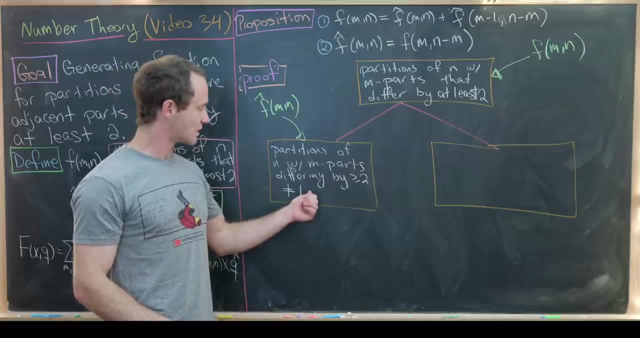 this next one down. But what we can do is talk about what is not in this orange box, And that's exactly what we'll do. So let's go over here and we'll describe the complement of this orange box. So this will be. 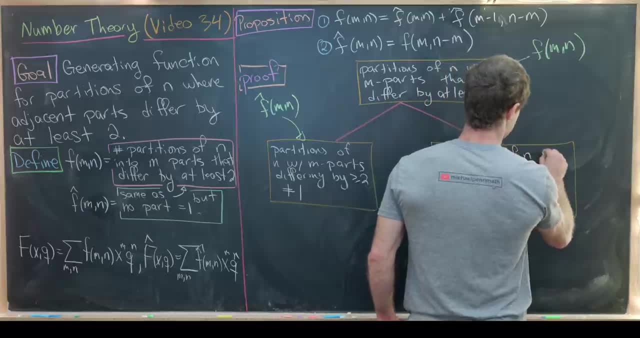 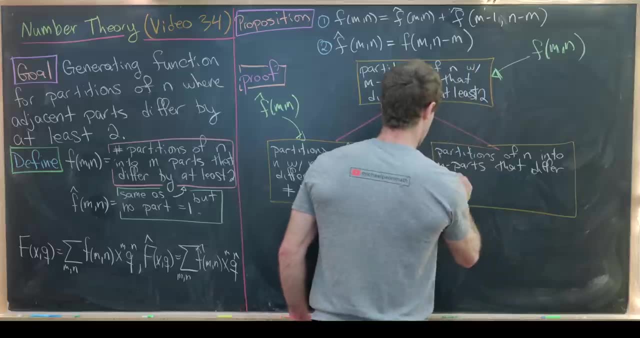 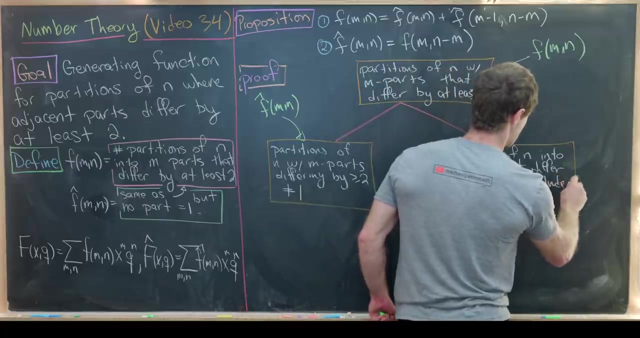 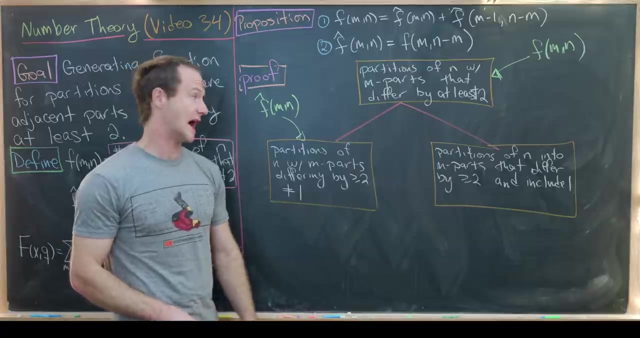 partitions of n into m, parts that differ by bigger than or equal to two, and they include the number one. So that means each partition in this box has the number one as the first part. Notice, it can only be the first part if it satisfies this rule. 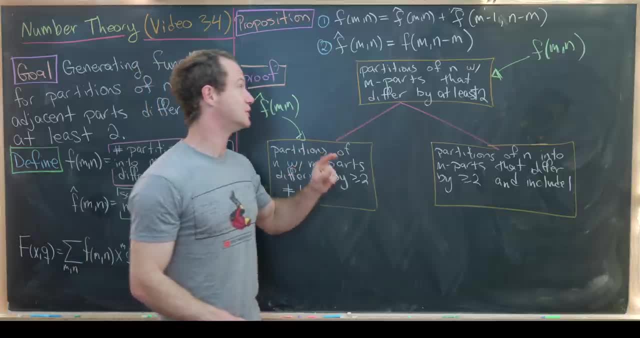 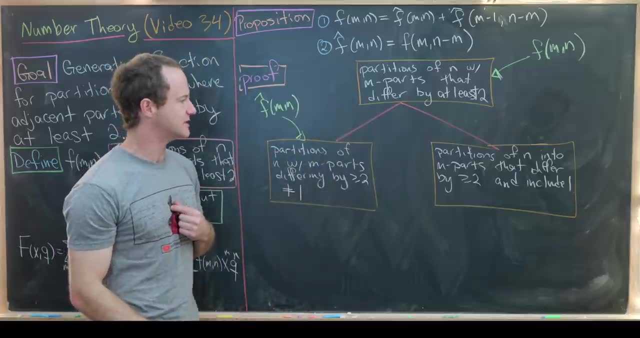 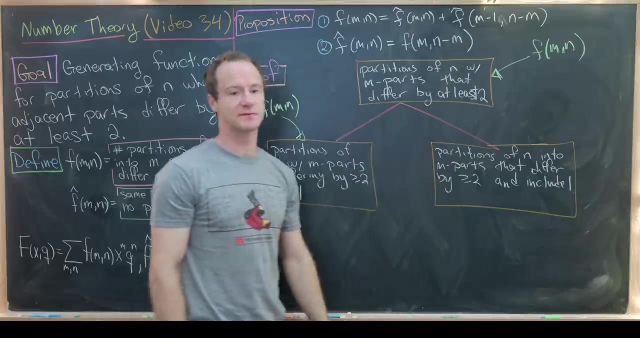 So I would suggest a nice, doable exercise would be to pick a value of n and m and fill all of these boxes in. Okay, so now what can we do? We want to somehow translate these types of partitions into partitions that are being counted by this function, And that's not too hard. So what we'll do is subtract. 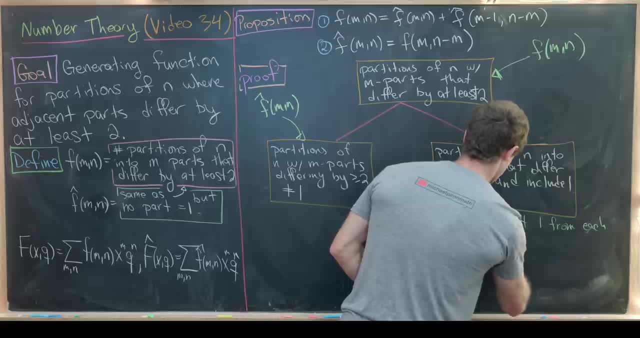 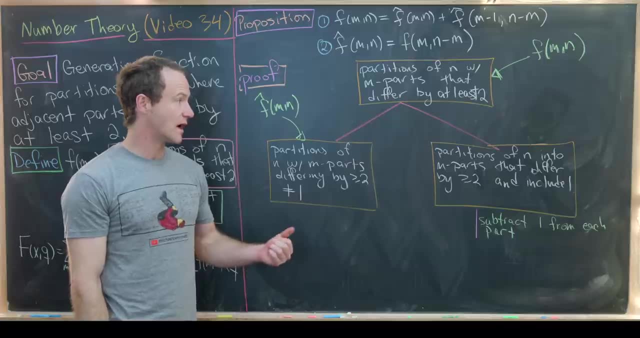 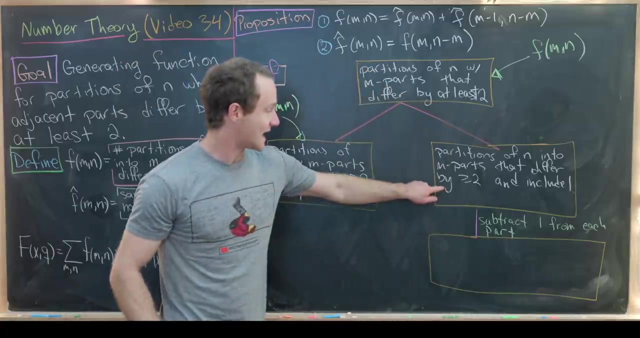 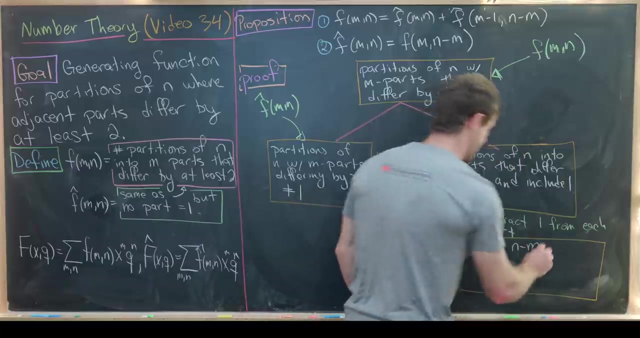 one from each part. Okay, So that means that we're eliminating the last part and then we are decreasing n by m. Okay, so let's see what effect that will have. So that will assign each partition up here to a partition of n minus m. 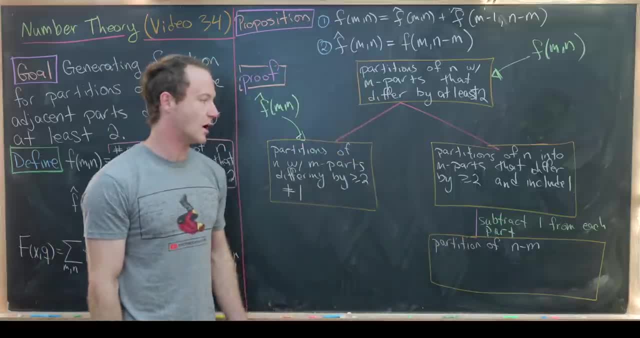 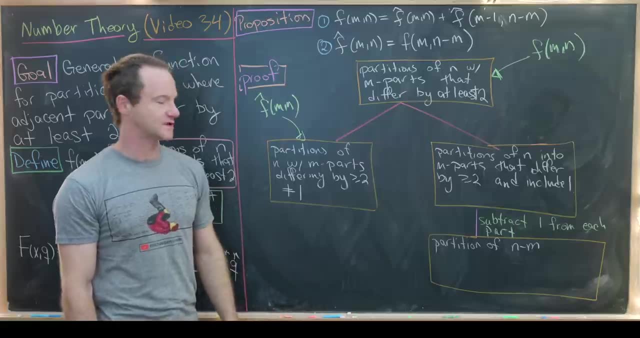 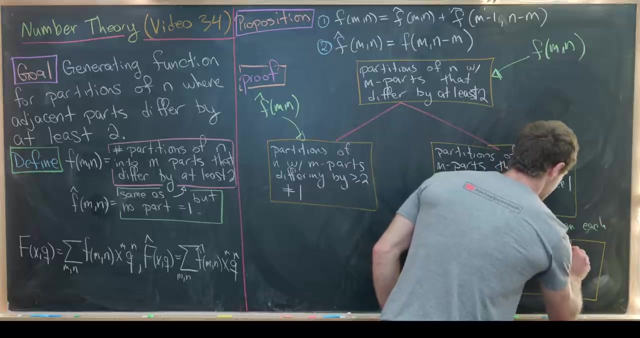 Well, why do we have to subtract m here? I just said we subtract one. Well, we are subtracting one from each part and there are m total parts. So that means all together we're subtracting m and then, furthermore, because we're subtracting from each part, they still differ by at least two. 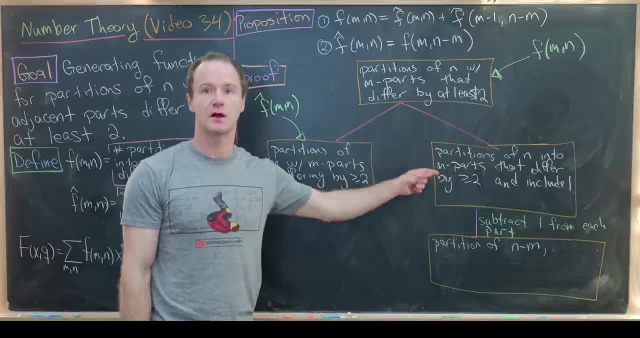 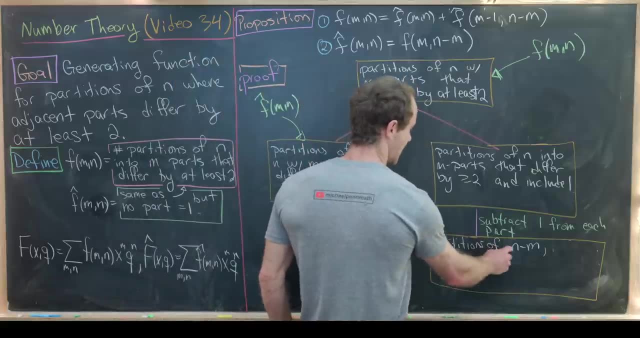 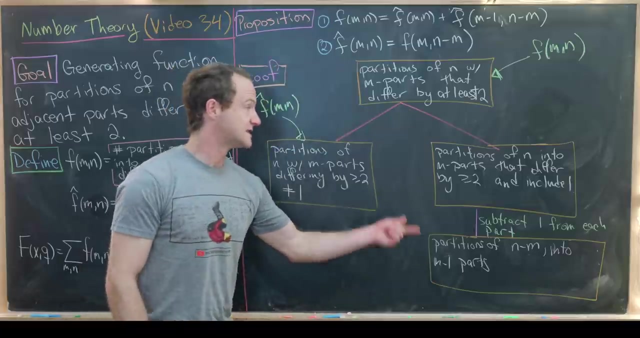 But now, since one was definitely one of the parts up here and we subtracted one from each part, that means we've decreased the number of parts by one. So this is partitions of n minus m into m minus 1 parts, And then we subtracted one from every part. this rule is still satisfied. So in other words, all. 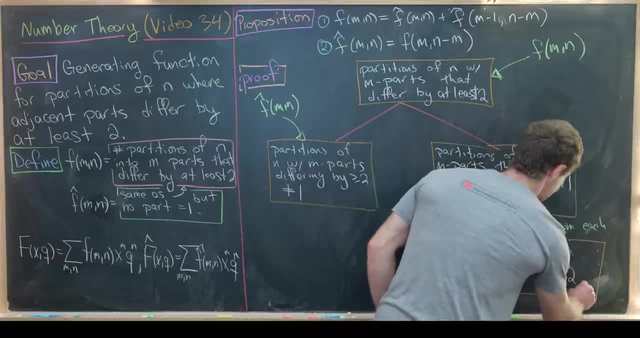 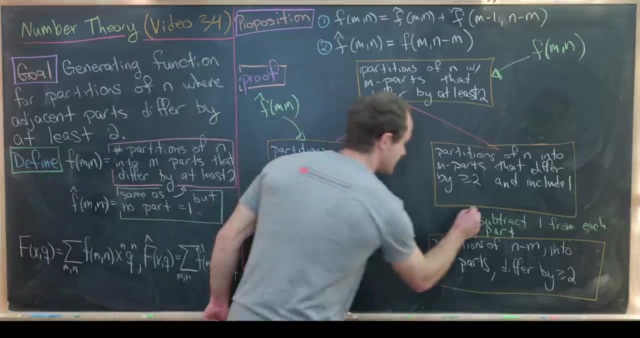 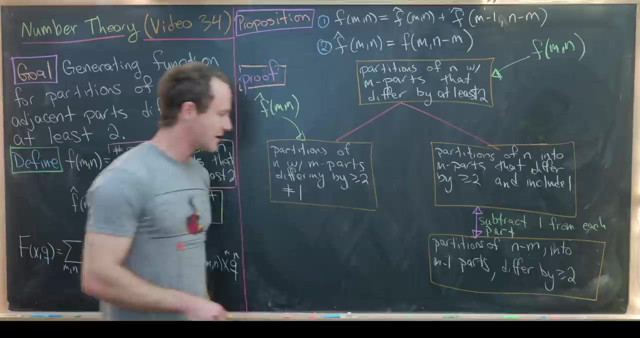 of these differ by at least two. The parts differ by at least two. So I think it goes without saying, or maybe it's a pretty easy thing to see, that this sets up a one-to-one relationship between the elements in each of these boxes. So now all we have to do is 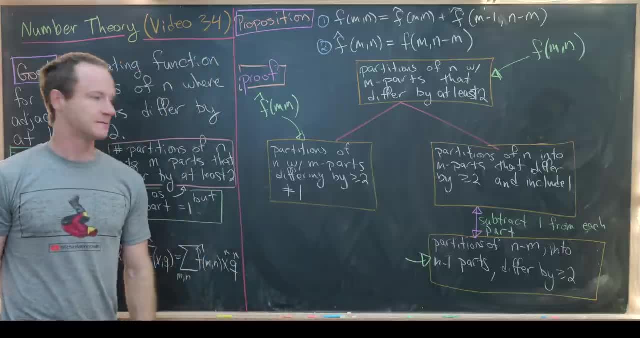 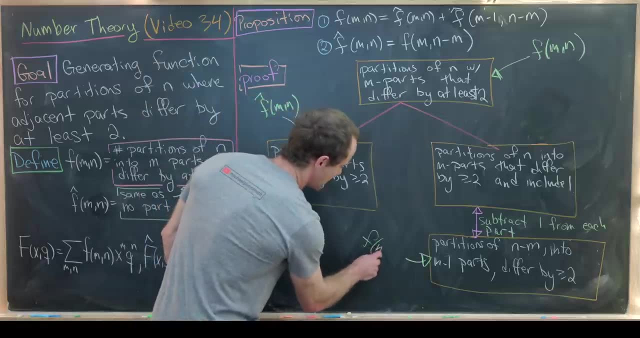 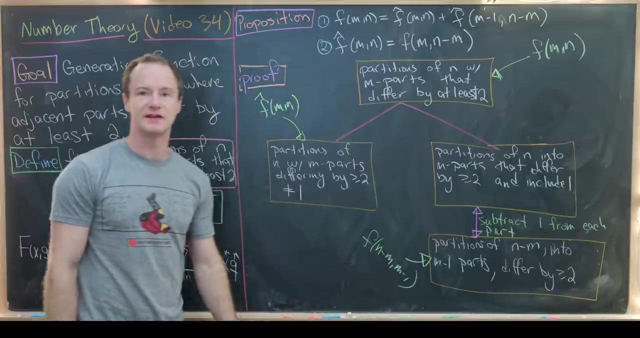 count how many guys are in this box, But that's not too hard because we've got a function that counts that exactly, And that is f? n minus m, m minus one, In other words, partitions of n minus m into m minus one parts. But notice, we almost have everything we need to build. 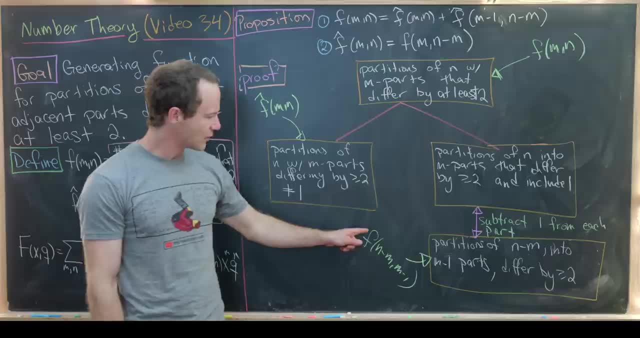 this equation. we just need a hat over this. So how can we argue that there's a hat over this? In other words, that none of these parts are in this box, So we just need a hat over this. So how can we argue that there's a hat over this? In other words, that none of these 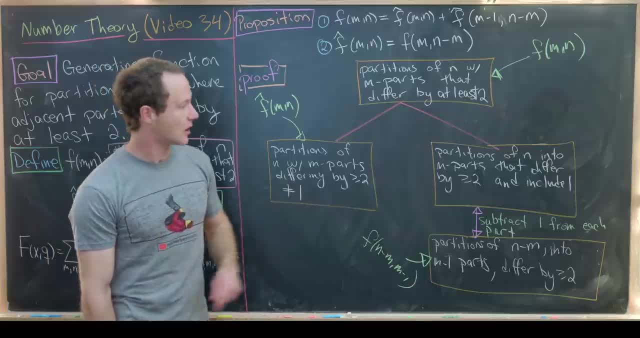 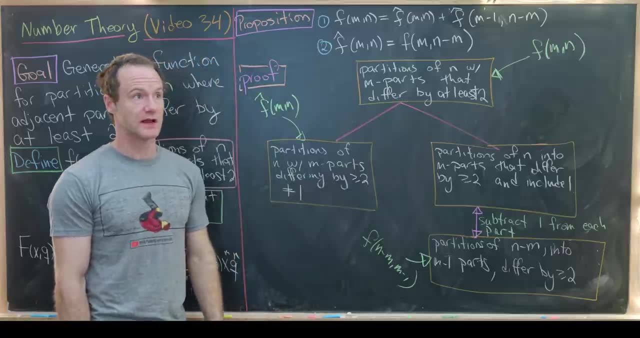 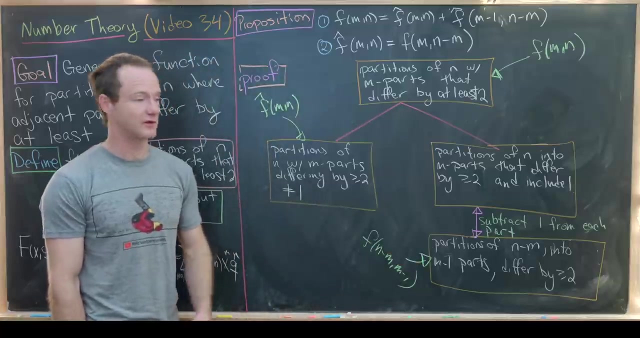 parts include one. Well, that's not actually that hard, because here every partition includes the number one, which means the second smallest part is bigger than or equal to three. So when we subtract one from each part, the smallest part down here will be bigger than or equal. 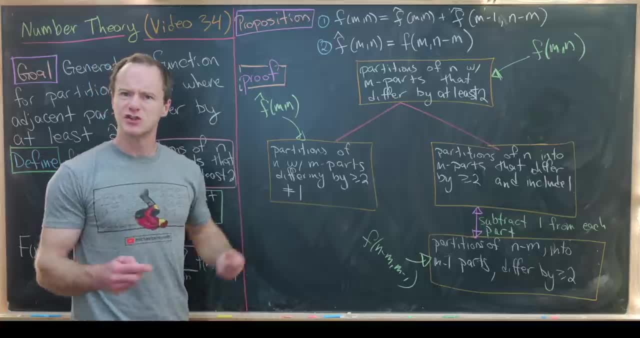 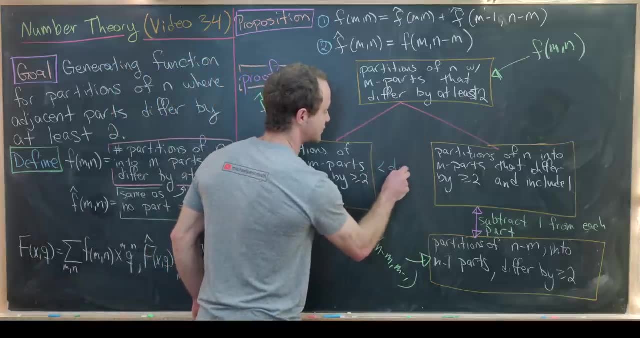 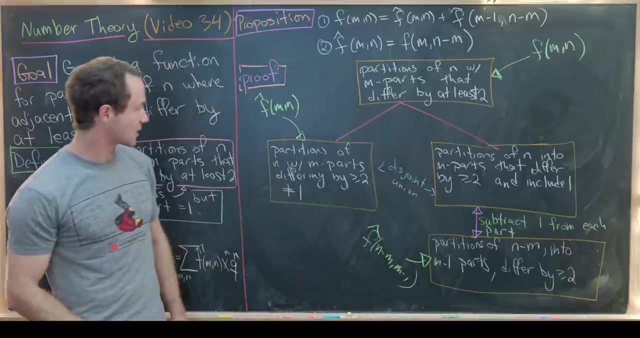 to two, So it will not include one. So by those rules I've just said, that means we can put a hat over this. But now what we've done is created some sort of disjoint- Yes union- of our set at the top into these two sets here which have f hat m n and f hat n minus m. 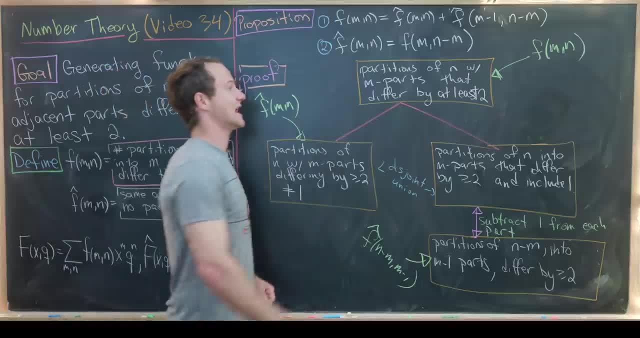 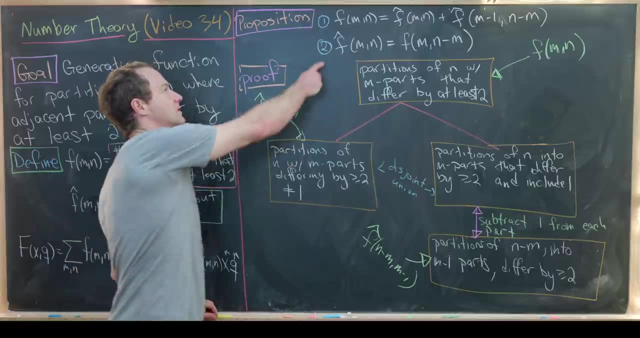 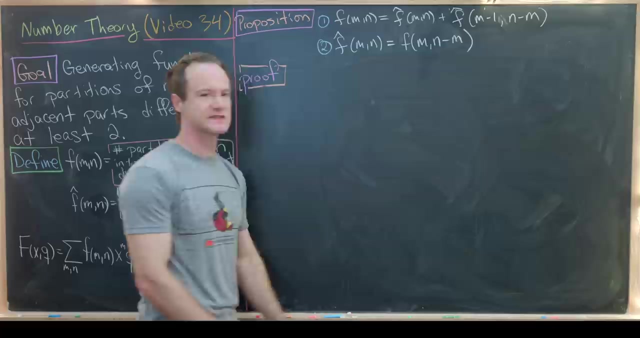 m minus one elements, whereas our original set had f of m n elements. So that builds this first equation. Okay, so let's maybe get rid of this and then we will build the second equation. We just got done proving this first equation. Now we're ready to prove this second equation. So let's see. 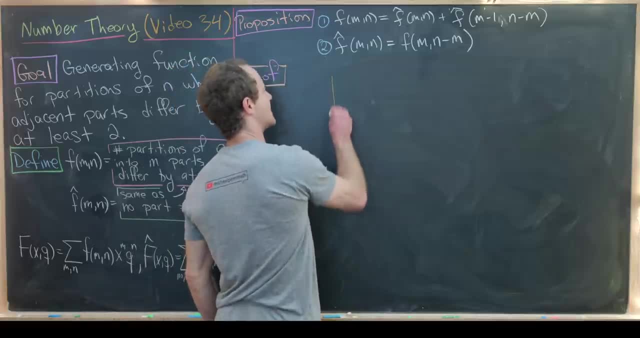 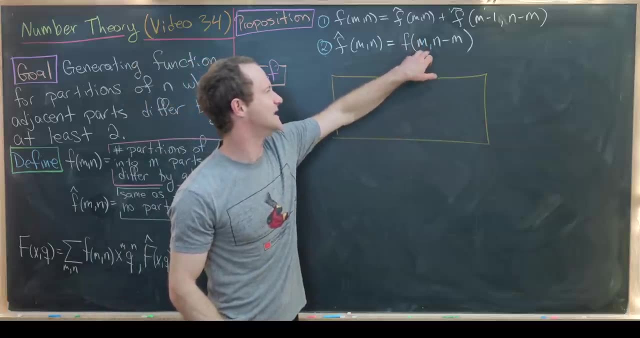 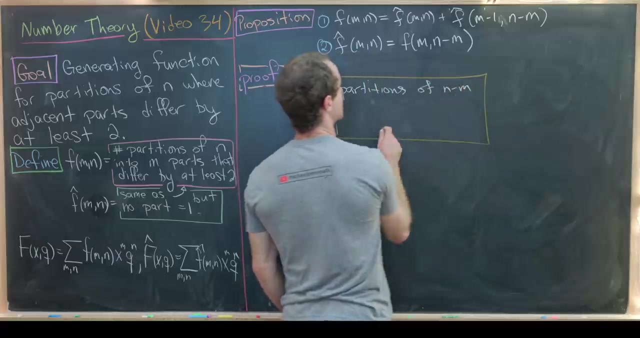 how we can do this. We'll do a similar strategy where I make a box where I put all of the partitions of a certain type. So I want to count up the number of partitions that this function represents first. So these will be partitions of n minus m, with m parts, and maybe this goes without. 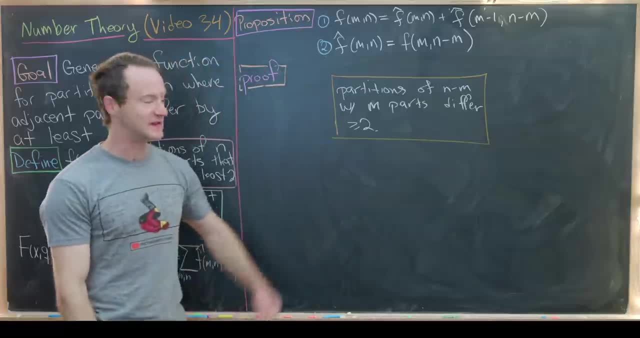 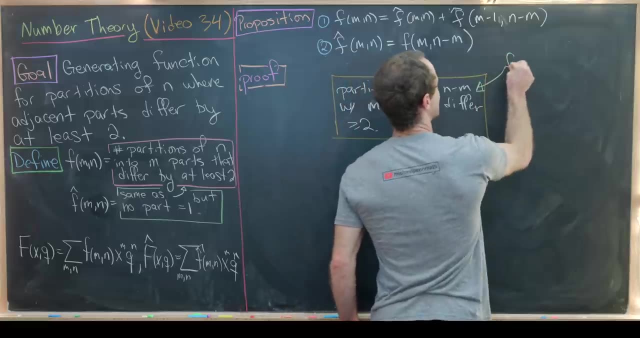 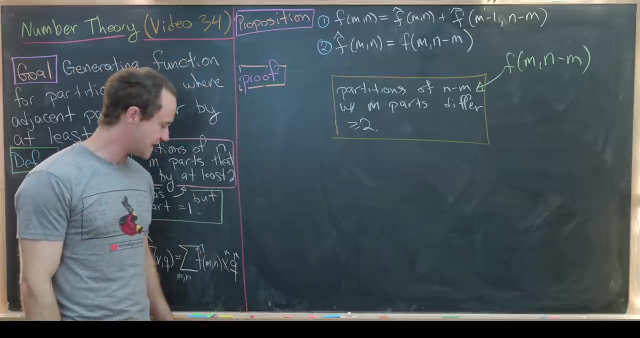 saying, because this is the whole world that we're living in in this video, but these parts differ by at least two. So how many elements are in this box? Well, there are exactly f, m, n minus m elements in this box. Okay, what will we do here? Well, we're going to do a similar transformation to what we did on the 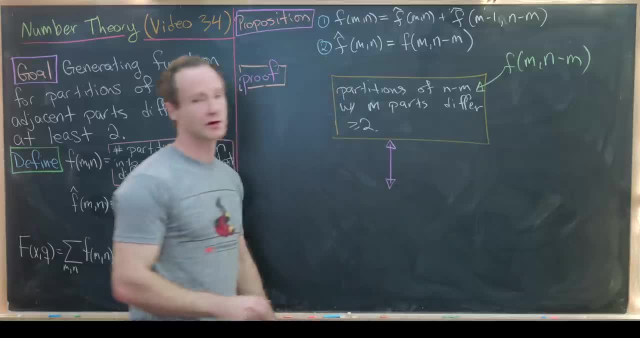 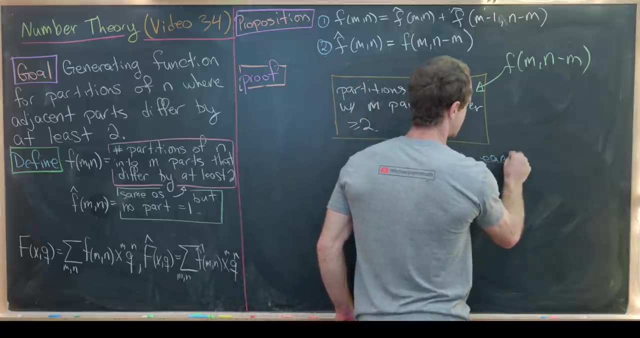 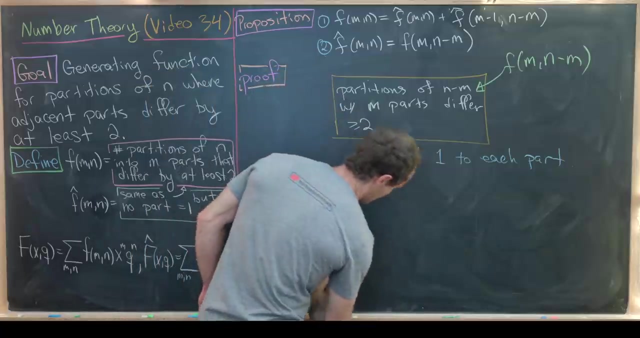 last board. So I'm going to set up this one-to-one correspondence, which is generated by adding one to each part of every partition in this box. Okay, so let's see how we can do this, So let's see what effect that will have. So that's going to give us partitions. 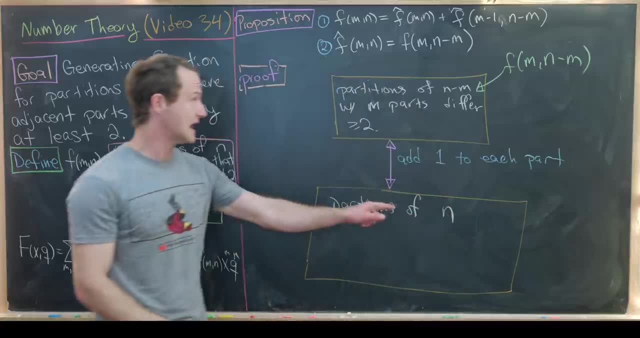 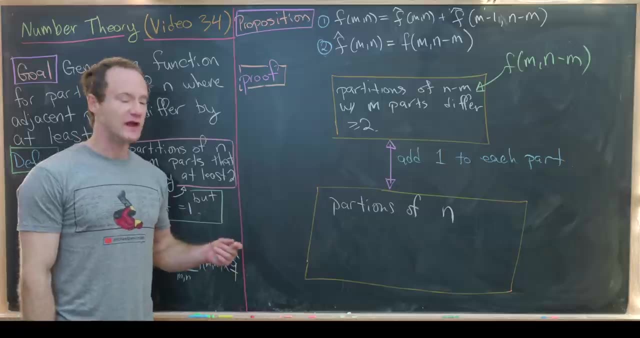 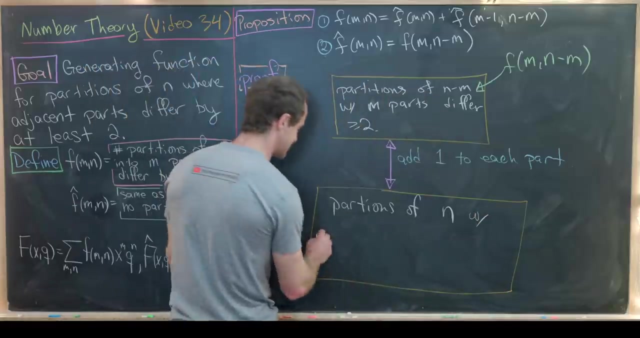 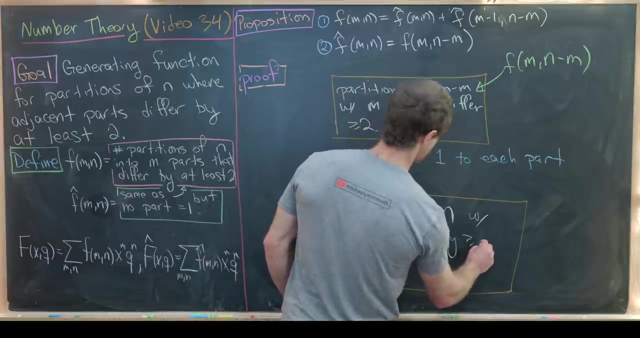 of n instead of n minus m, because we've added one to each of the m parts. So in the congregate we have added m, but we have not changed the number of parts. So this is still with m parts. They still differ by at least two. 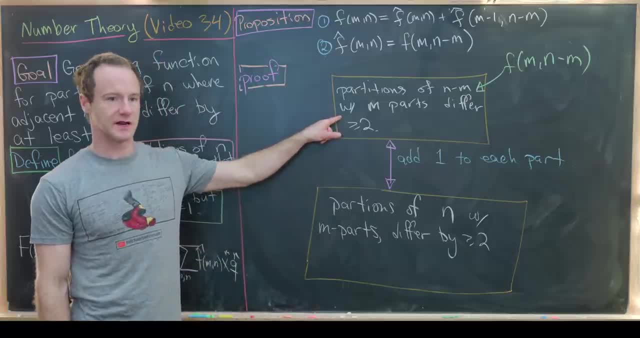 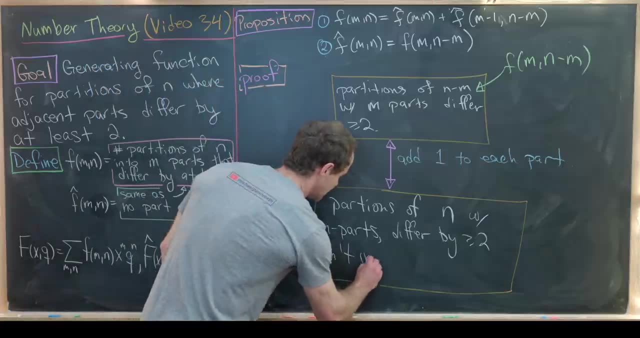 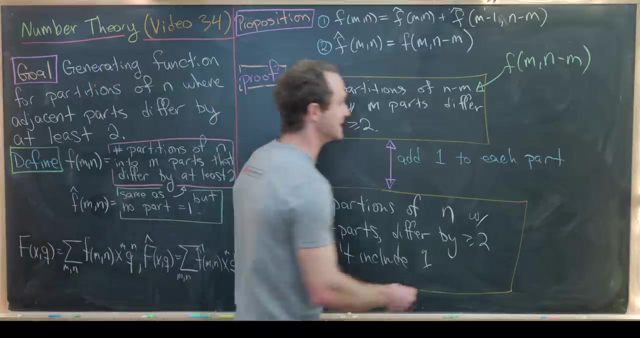 And furthermore, since one was the smallest possible part here, the smallest possible part down here is one plus one, So that means these don't include the number one. Okay, but now we can easily count up the number of partitions in this box, and it's exactly what we want it to be: It's f? hat m? n. 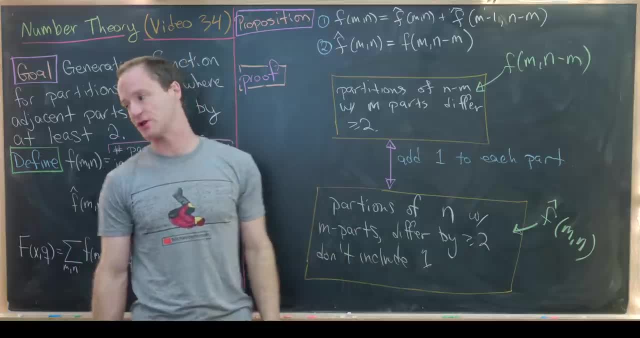 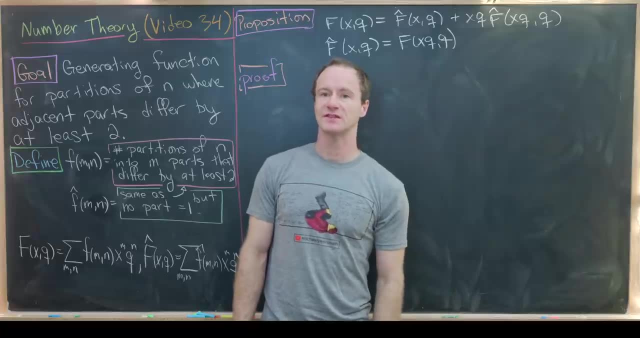 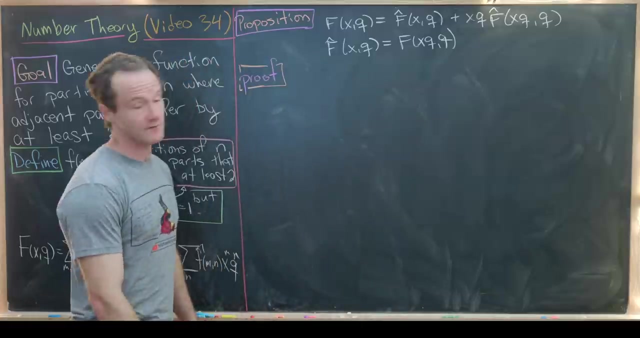 Now we're going to take this result and write a generating function version of it, In other words, a version of it that involves these capital f and f hat functions. We just got done proving a nice recursion for these functions- little f and little f hat- And now we want to look at a generating function version of those. 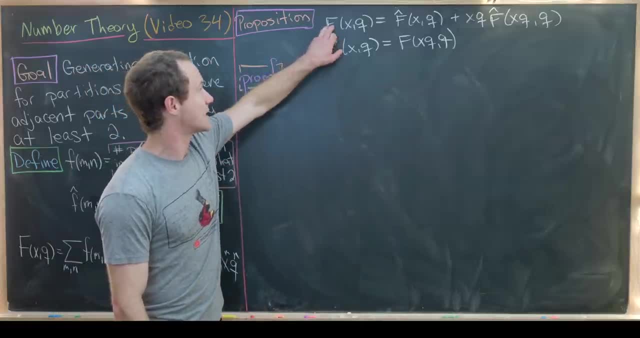 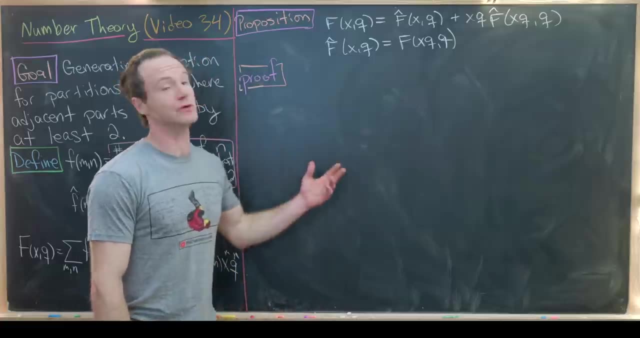 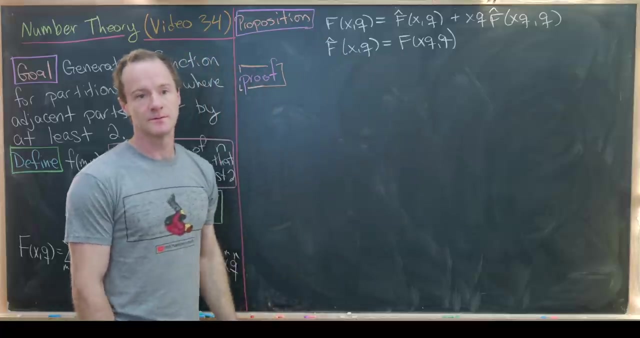 recursions. So we've got this first one: capital f of xq is equal to capital f hat of xq plus xq capital f hat of xq q. And then the second one: f hat xq is equal to f xq q. So let's start with. 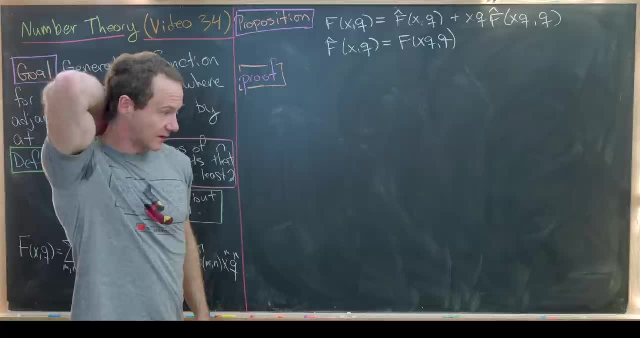 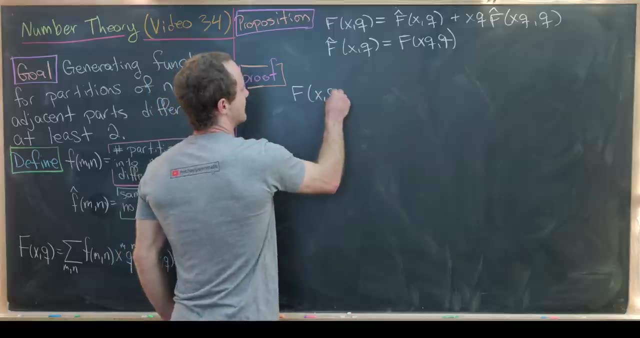 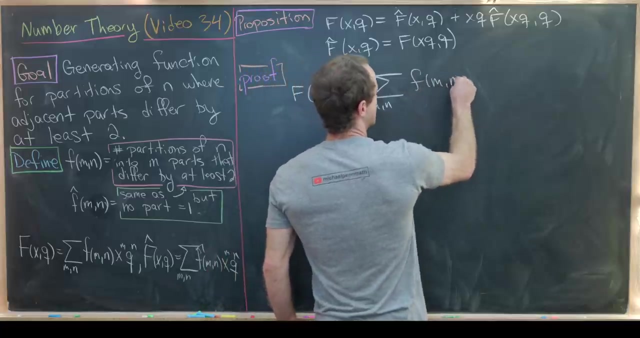 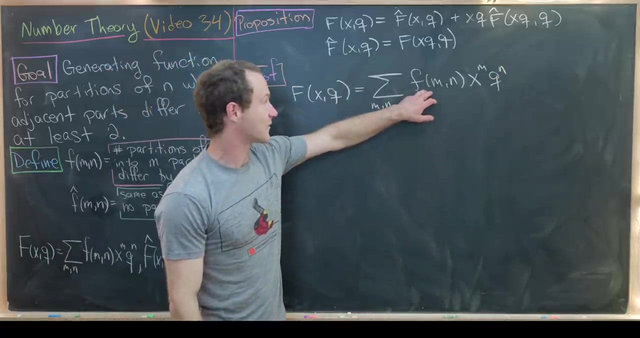 this first one, And as we'll see, these follow pretty quickly from the recursions that we just got done proving, So we'll start with the left hand side of this. So we have: f of xq is equal to our sum over m n of f, of m n. x to the m, q to the n. Nice, Now we'll apply our first recursion to. 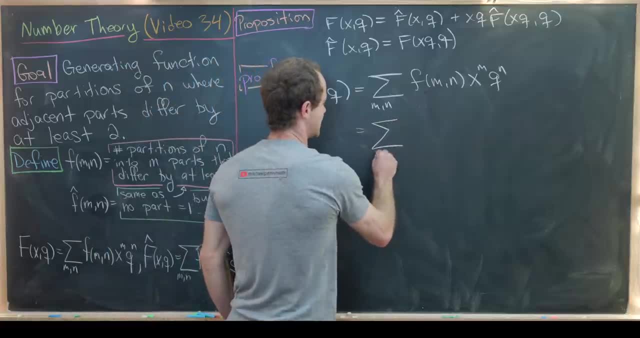 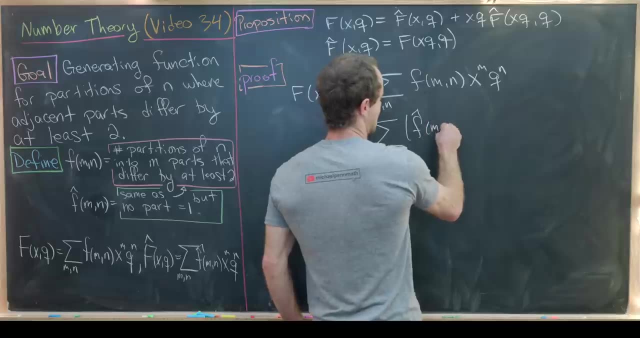 this little f m n. So that's going to give us this sum as m n x to the m, q to the n, And then we'll notice that m and n go between zero infinity, although I'm leaving that off of f hat m n plus. 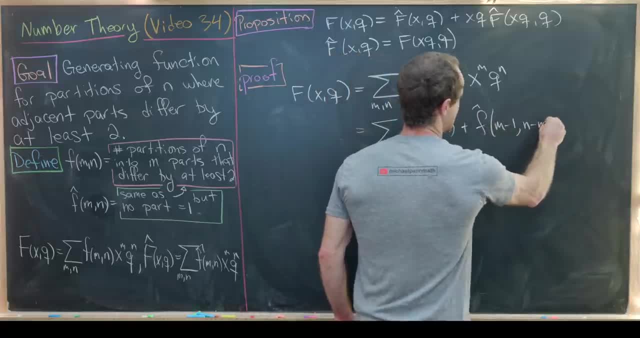 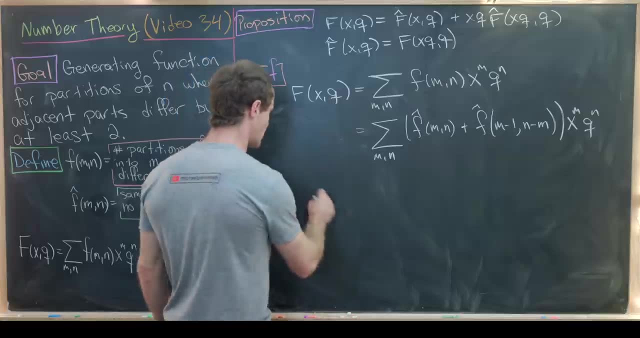 f hat m minus one, n minus m. Then we've got x to the m, q to the n, like that. Now we're going to split this into two parts, So that's going to give us this sum, as m and n go between zero and. 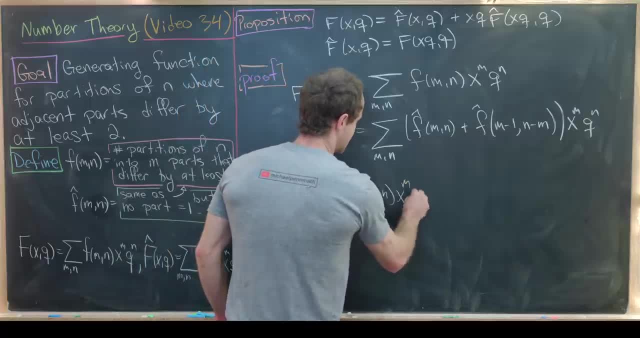 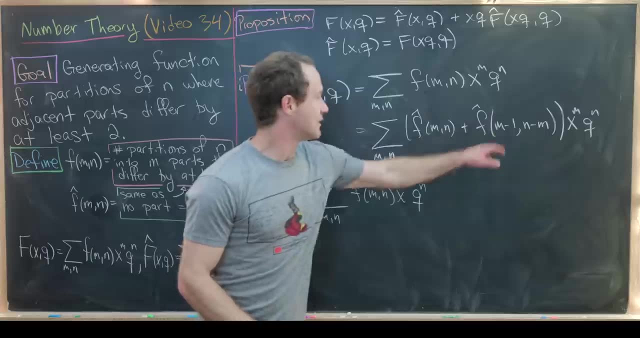 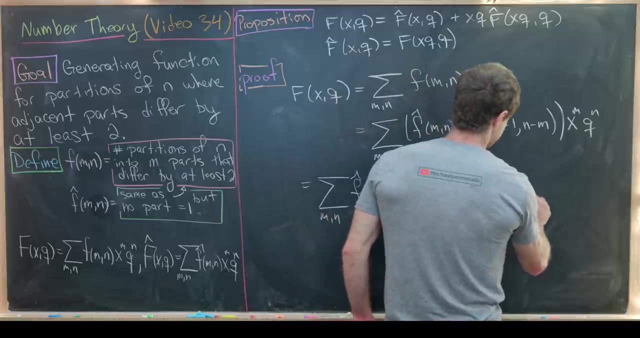 infinity f hat, m, n, x, m, q to the n. So notice, that is all the sum that we've got. So we've got already our generating function, capital f hat, And then we've got the rest of this. So that's going to be plus our sum over m and n of f hat, m minus one, n, minus m x to the m, q to the n. 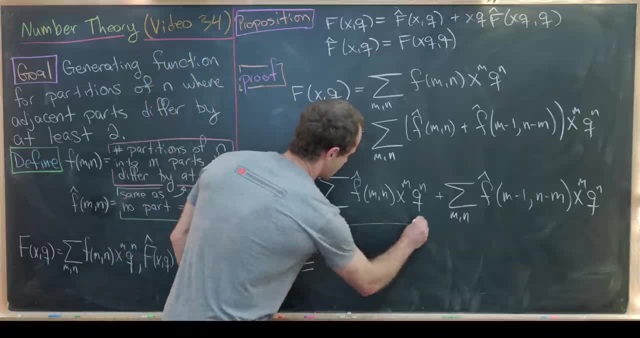 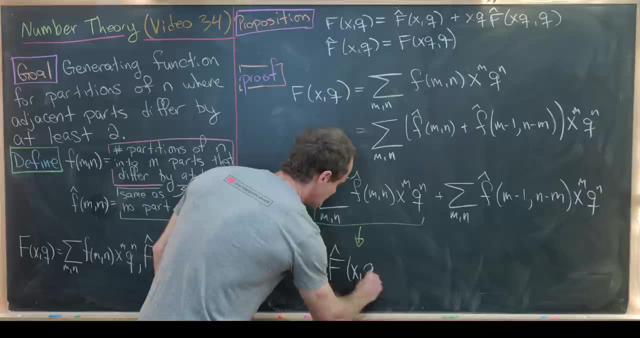 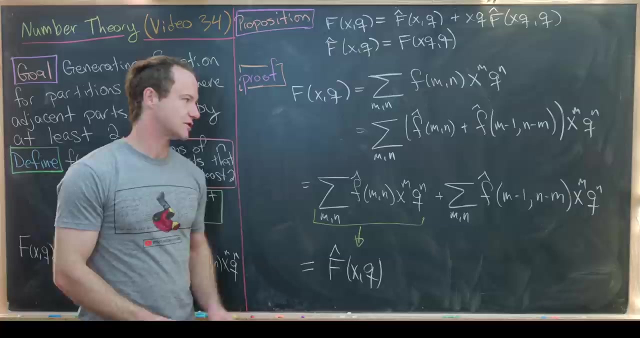 So, like I said, this guy right here looks exactly like our f hat generating function already. So I'll just rewrite this as f hat, x, q, And then we can get to work on this other bit, which will be a little bit of re-indexing. So let's see how we might want to re-index this. Well, I think. 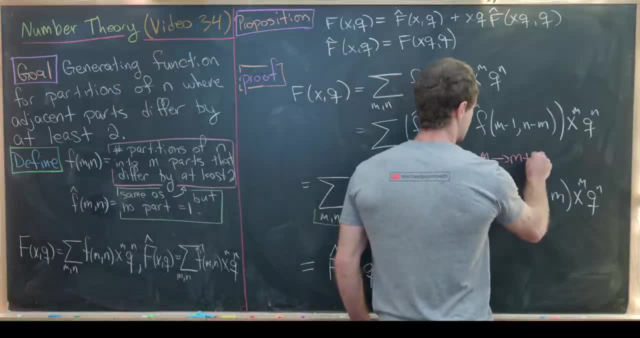 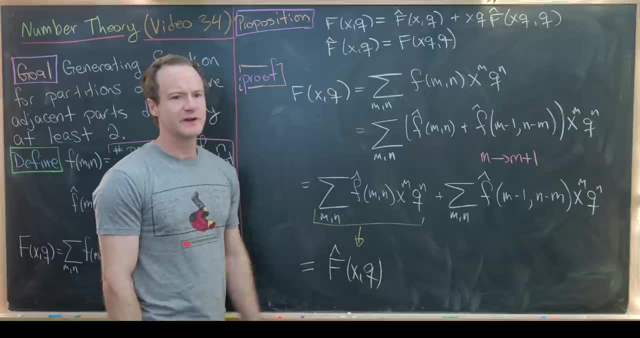 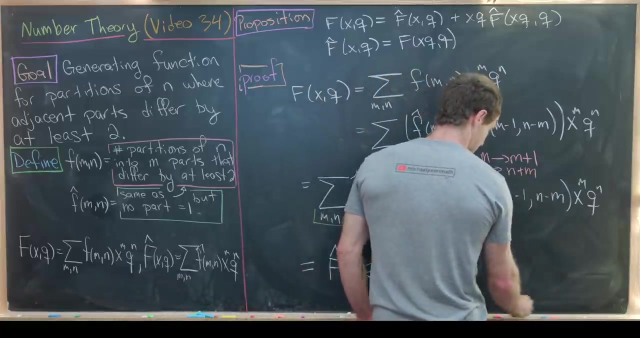 probably our best bet will to send m to m plus one. So in other words, we're going to replace all of the m's with m plus ones. And then what should we do with the n's? Well, we're going to send all of the n's to n plus m. Now you might be a little bit worried about what's happening, kind of. 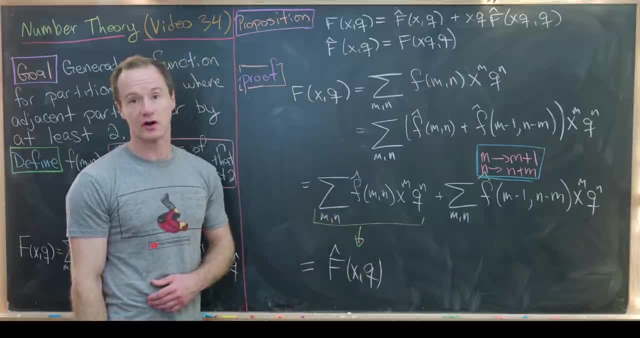 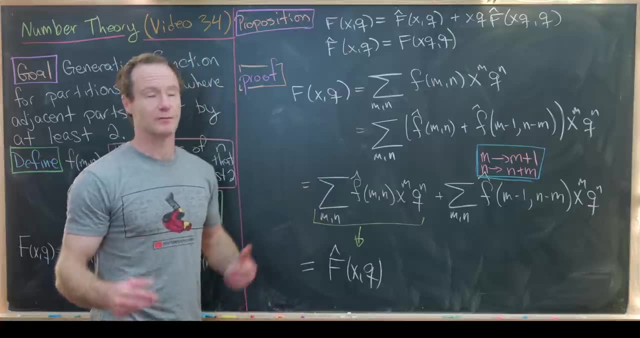 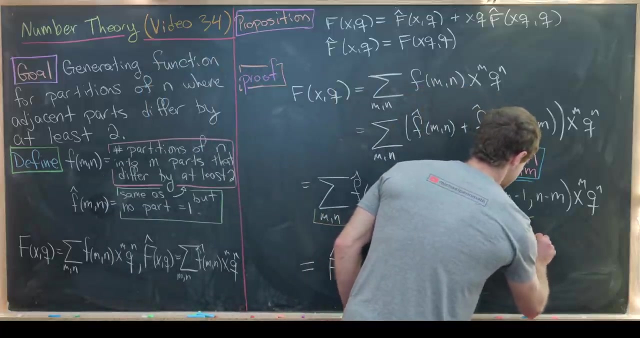 at the lower end here because we have to change the starting point. But I'll let you guys think about why. that is not a problem. We're essentially just counting and leaving out a bunch of zeros, So how does that allow us to rewrite this guy? That allows us to rewrite this guy as the sum. 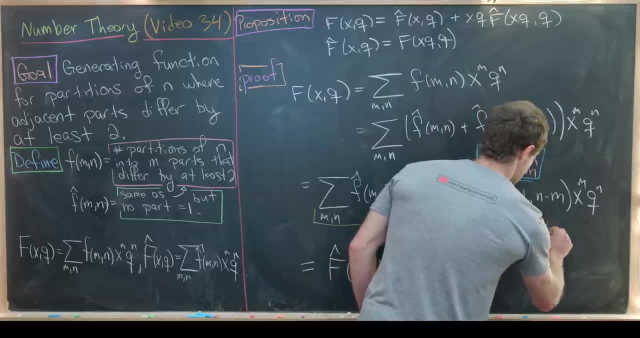 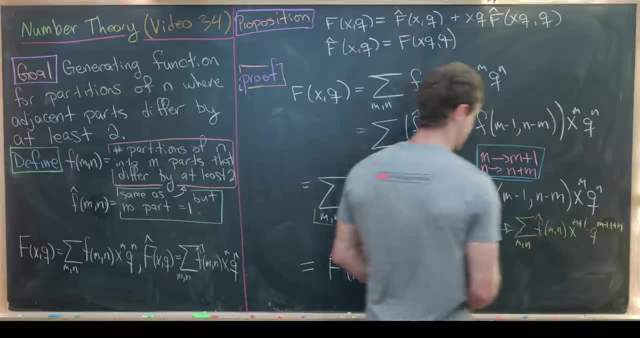 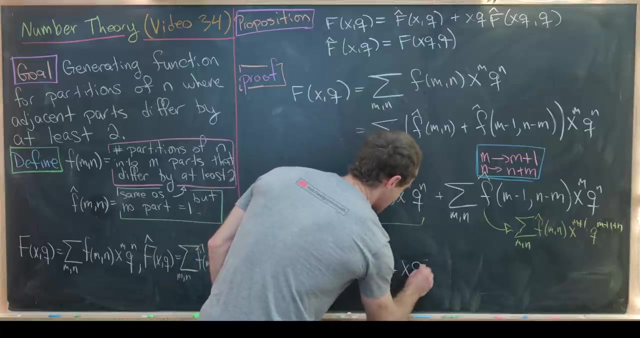 over m? n of f hat m? n, And then we'll have x to the m plus one, q to the m plus one plus n. Let's factor some stuff out of this and rewrite it a little bit. So this is going to be x times q. 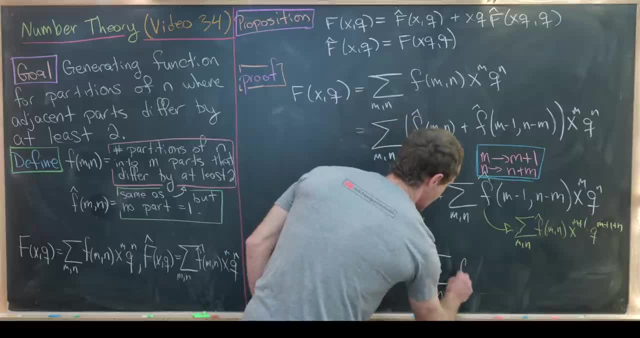 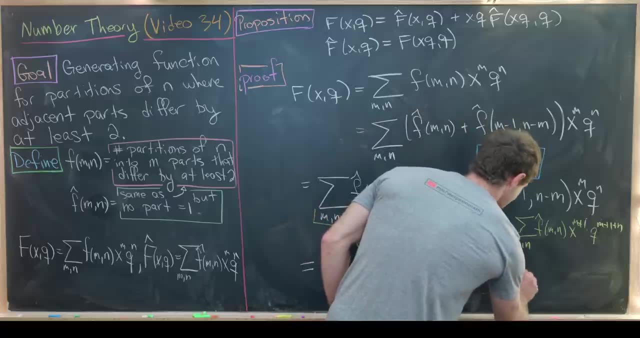 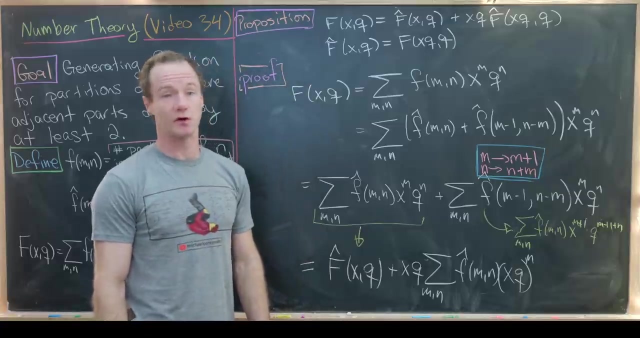 times our sum over m n of f hat m n And then what's left over after we factor that bit out. So we will have x times q all to the m power. I've put those together just because that's what's being clued into us over there. And then we will have q to the n power. But let's notice that if 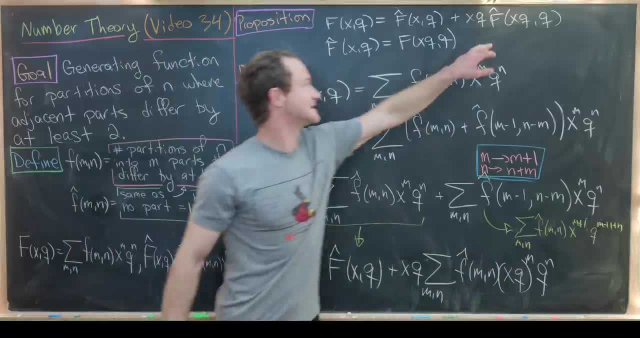 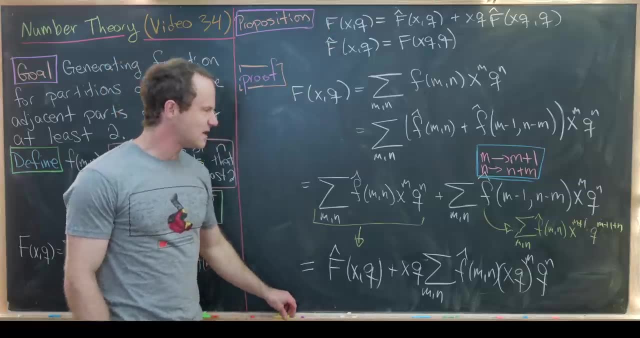 we rewrite this using our f hat generating function, it would be exactly this term right here. So that means we have proven this first identity And then maybe this second one is a nice one that could be left as a little bit of a homework exercise. It follows pretty similarly. 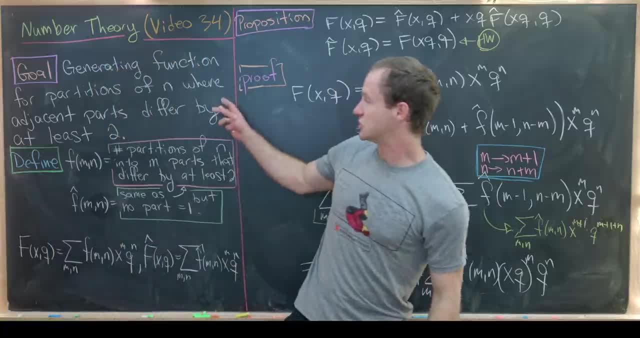 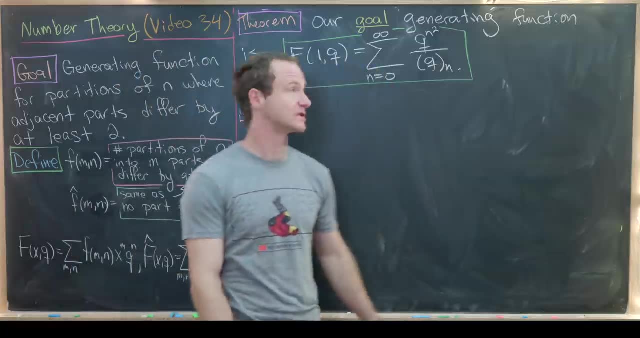 Okay. so now we've got everything in place to achieve our goal. Now we're ready to prove our goal, And that is the generating function for partitions with this restriction. So we've got f, hat, m, n, plus one q to the m power, And then we're going to have x times q to the m power, And 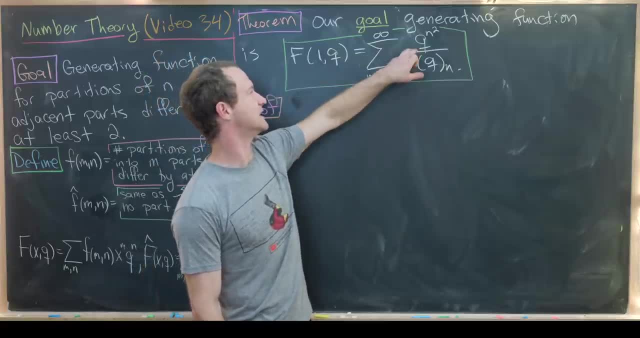 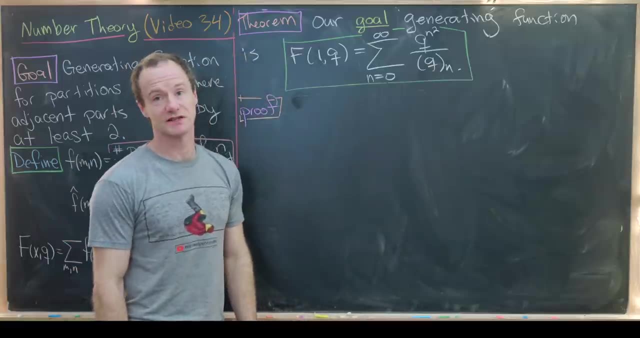 then we're going to have f of one. q is equal to the sum, as n goes from zero to infinity, of q to the n squared. And then this pockhammer symbol, q, n. So recall that's a product of n objects in the. 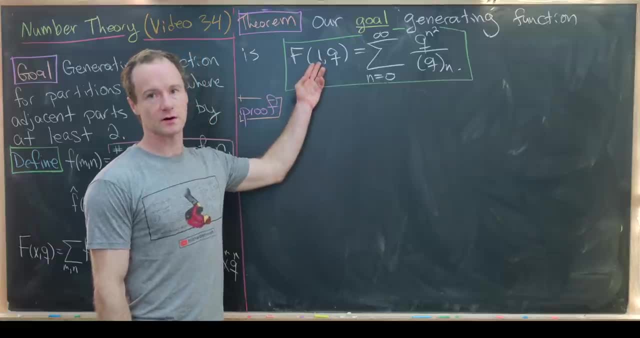 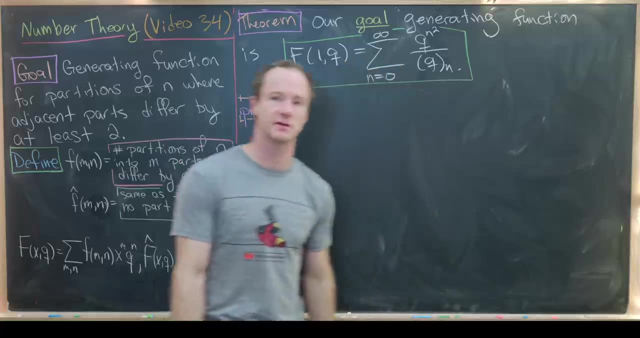 denominator. You might say: well, what's this one here? Well, the one allows us to count the number of partitions without worrying about this restriction on the number of parts. I'll let you guys think about that a little bit. Okay, so let's get to the proof. So, from the previous 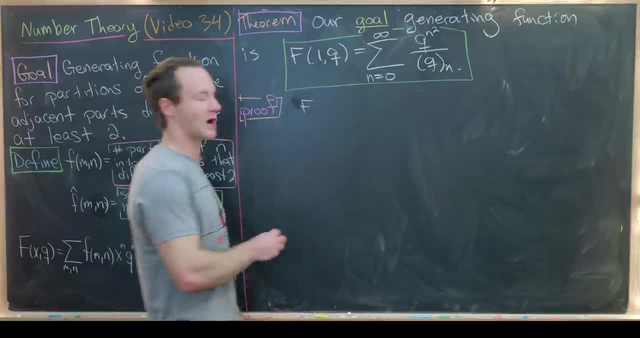 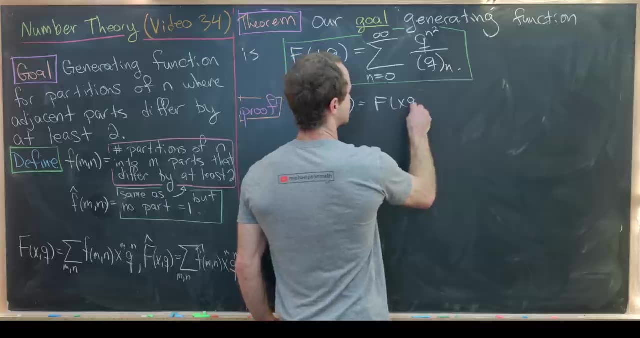 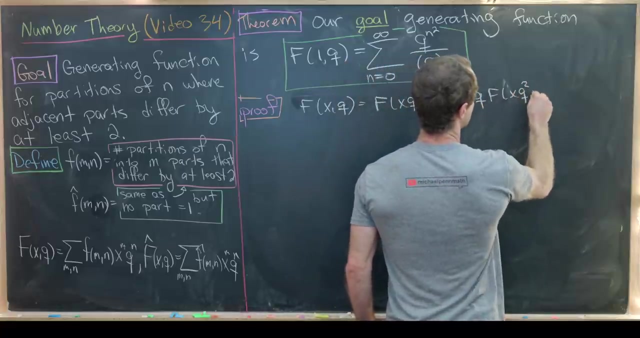 proposition. we can put those two portions together And then we can put the number of partitions of the proposition together into this single equation. f of x q is equal to f of x q q plus x q times f of x q squared q. So let's recall that the part that we proved had something. 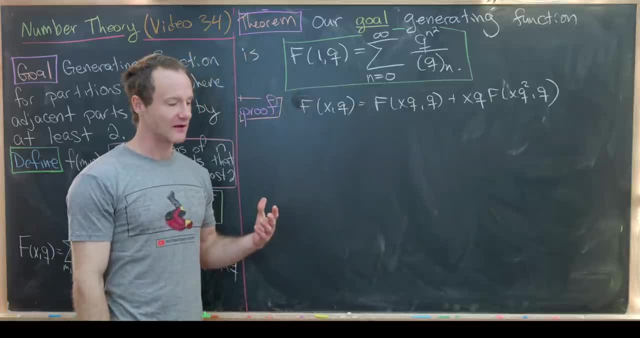 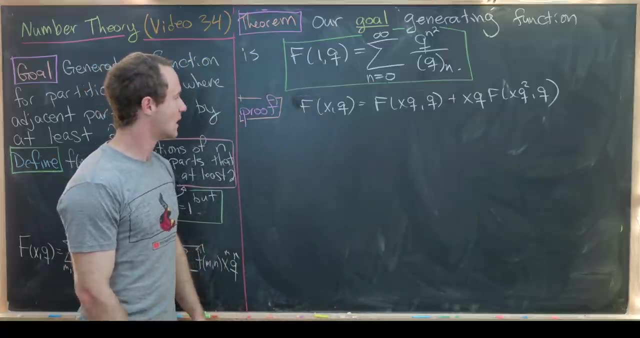 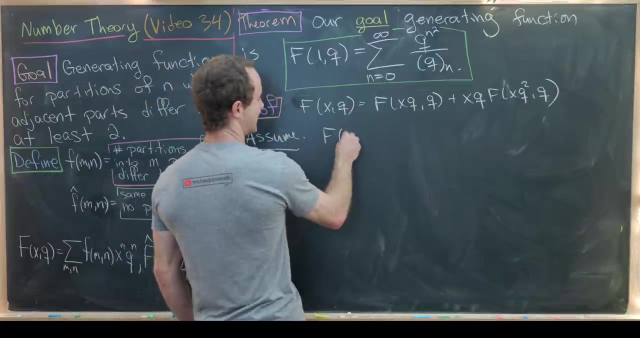 with hats over here on the right hand side, But the part that I left as homework would allow you to translate those into just the standard f's without the hats. Okay, so next we're going to assume that we have the following expansion: So f of x, q. 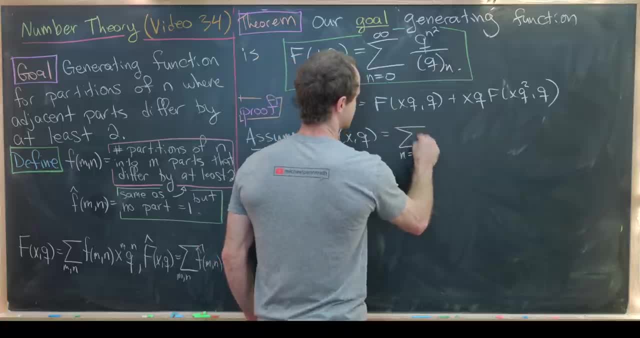 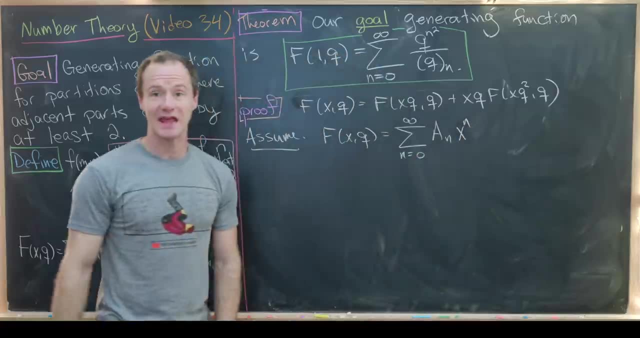 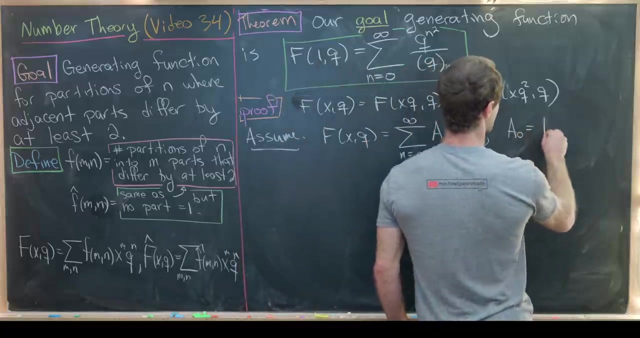 is equal to the sum- as n goes from zero up to infinity- of a n times x to the n. So those a? n's are going to all depend on q, And I want to point out that it's not too hard to see that a zero should be equal to one. Well, that would be like the number of partitions. 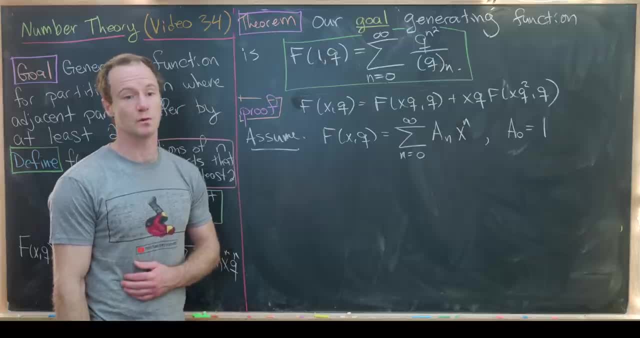 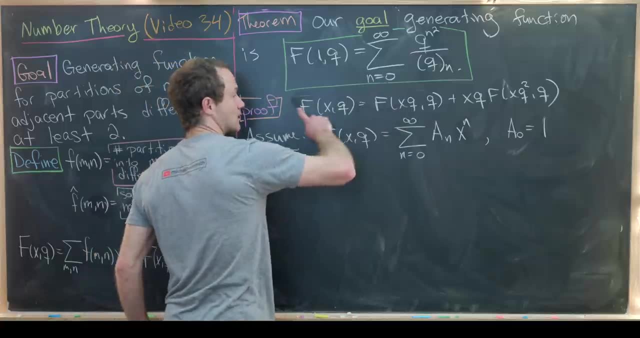 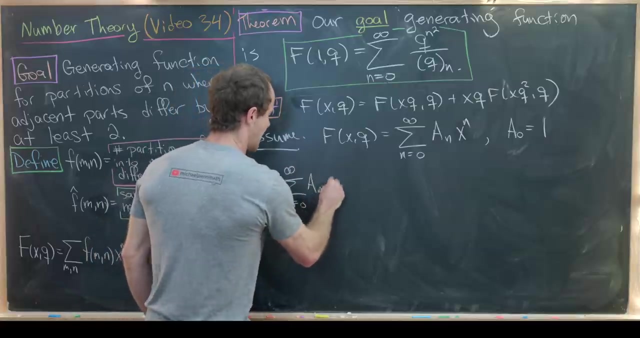 with zero parts, but we take things like that to be equal to one generally. Okay, so now we'll plug this expansion into our recursion or our difference equation up here, And that will give us the sum, as n goes from zero up to infinity, of a, n, x to the n equals the sum as n goes from zero. 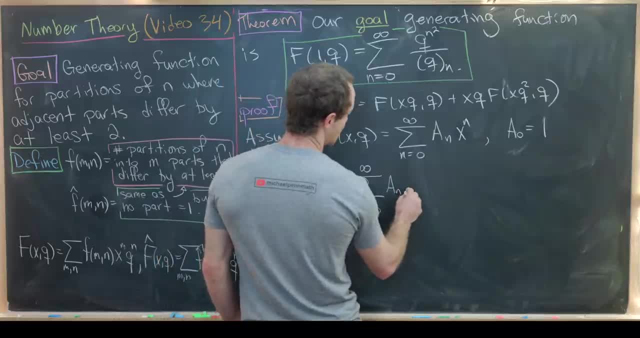 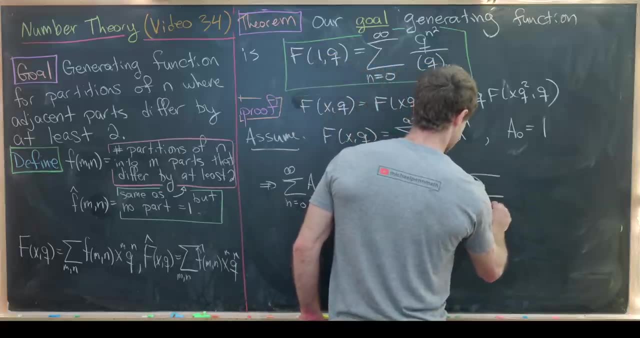 to infinity of a, n times q to the n, x to the n, plus a n times q to the n, x to the n. So that's x times q times the sum as n goes from zero to infinity of a- n. And then let's see what we've. 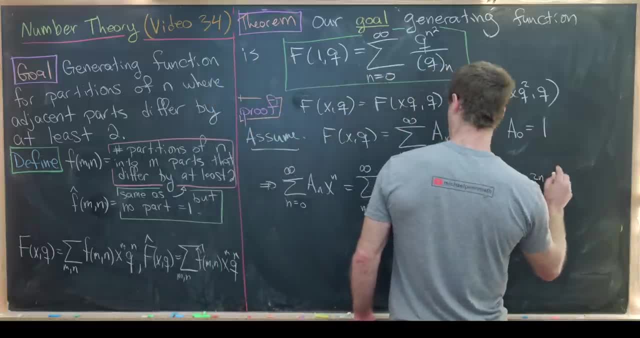 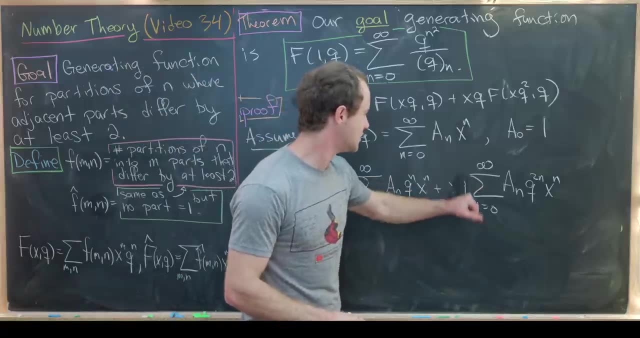 got here. We've got q to the two n and then x to the n, So we've got something like that. So next I'm going to take this x times q and bring it in. And we can bring it in by adding: 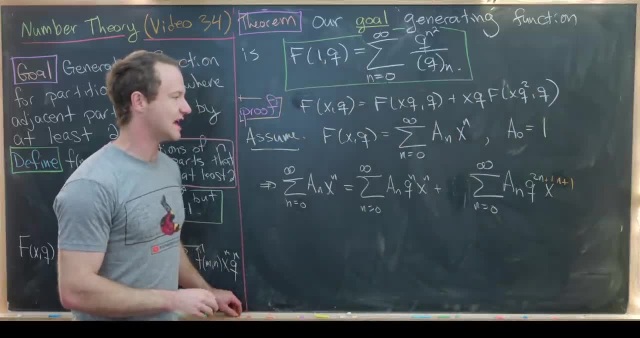 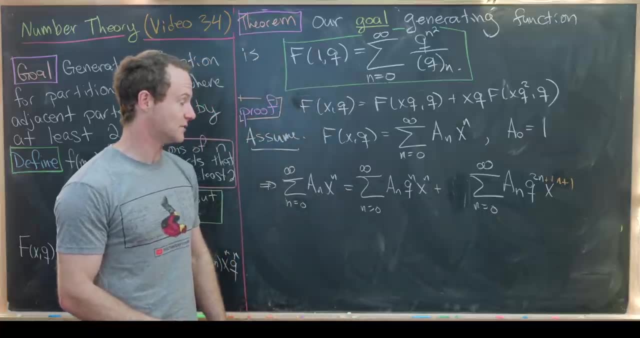 one to each of these exponents. So we have q to the n plus one and x to the n plus one. Next up, I will re-index this sum so that my x has an nth power. So I can do that by sending n. 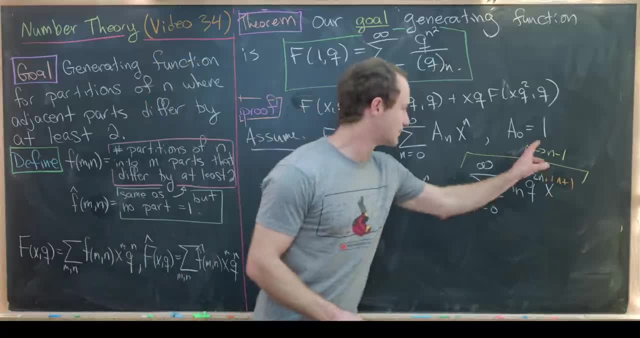 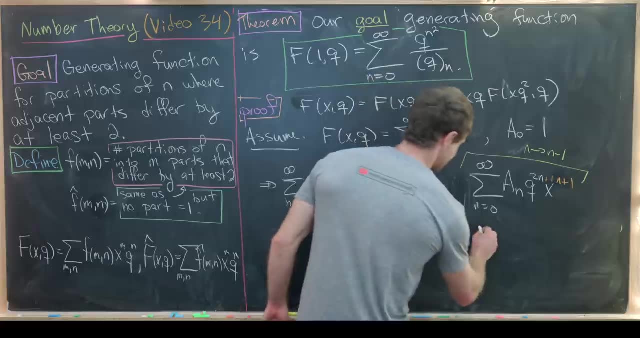 to n minus one. So that means n plus one will be. well, n minus one plus one, which is just n Okay, so let's see what effect that has. So that's going to give us the sum of a sub n minus one. 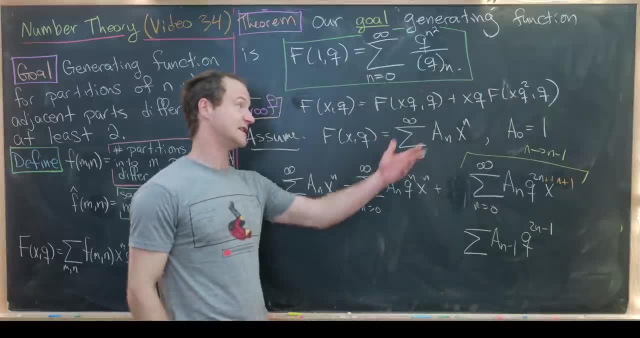 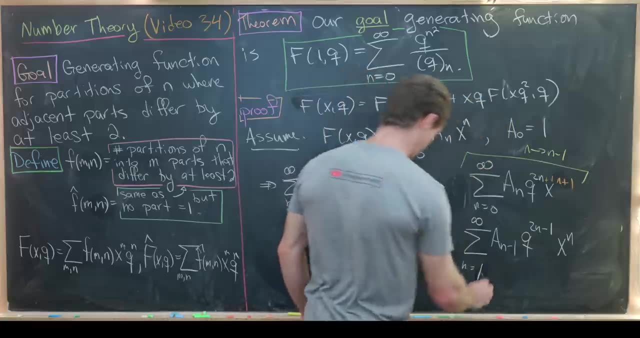 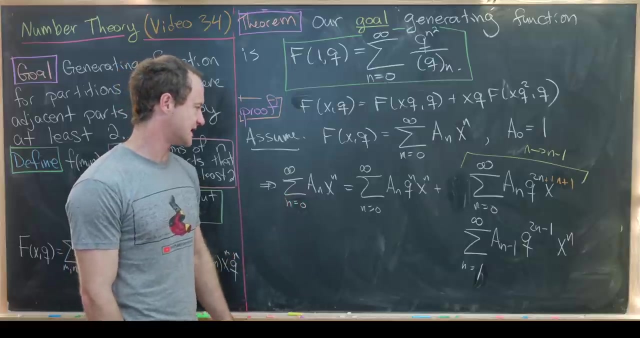 q to the two, n minus one. That's the effect if we replace n with n minus one. x to the n. But now this is just going to be the sum, as n goes from one to infinity because of our change to index. Next up, we can see that the only two constant terms in x are equal to one. 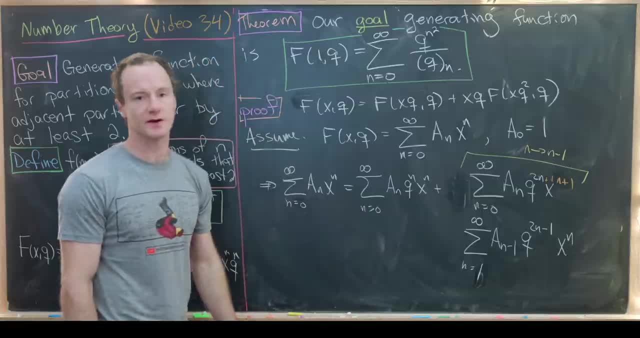 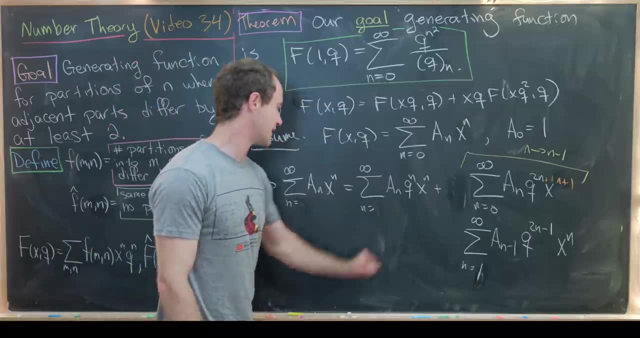 and they occur in this sum right here and this sum right here, So we can subtract a zero from both sides and that will change this from a starting point of zero to a starting point of one and likewise over there. So we're running out of room. 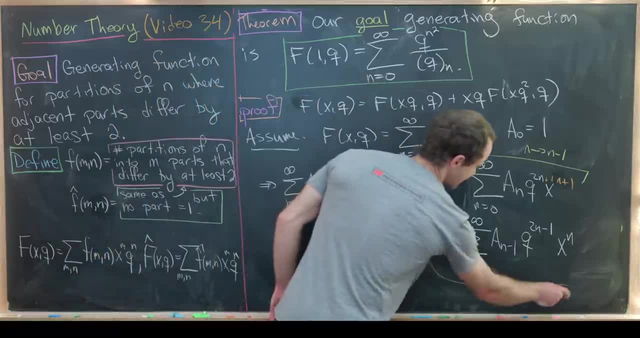 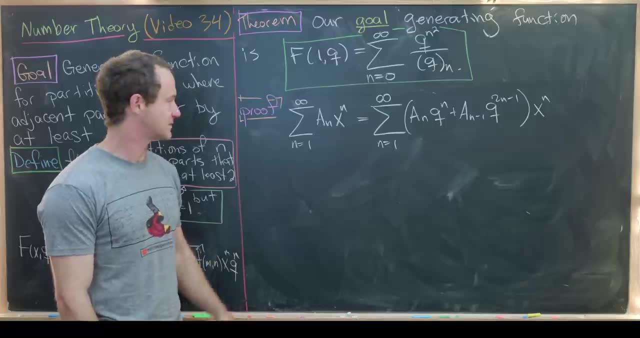 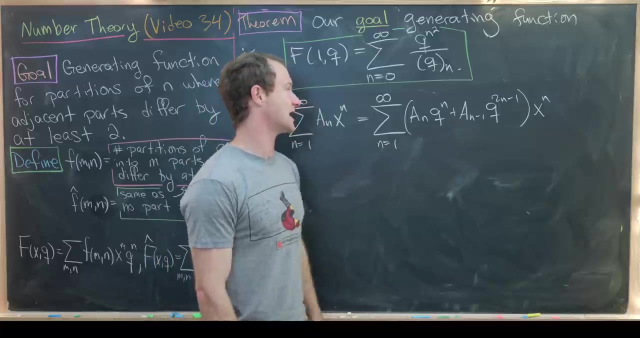 so what I'll do on the next board is rewrite this thing that I've underlined in yellow, and I'll probably push these two sums together. So after pushing the sums together on the last board, we have the following: So the sum of a n x to the n is the sum of a n q, n, a n minus one q. 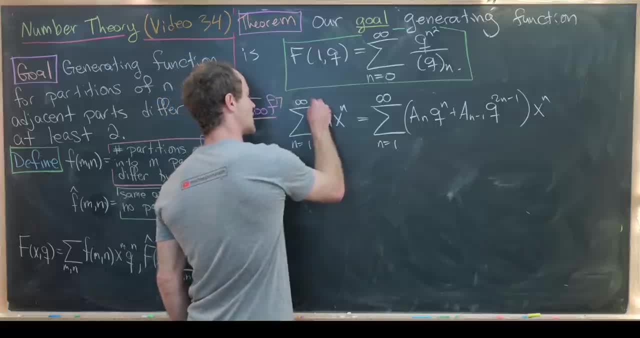 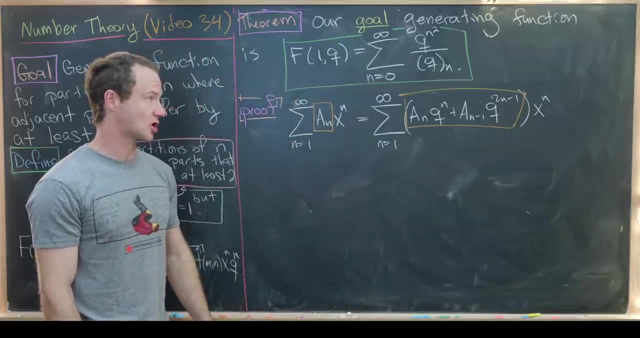 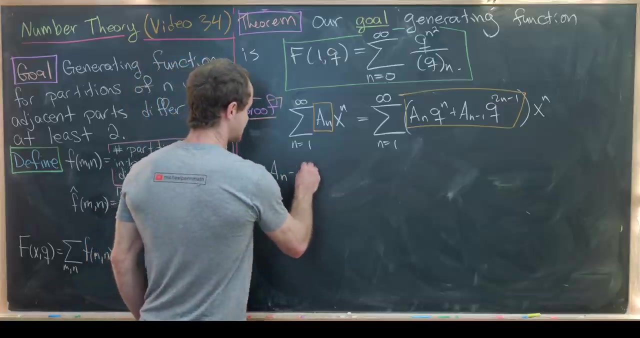 to the two, n minus one, x to the n. So now we can equate coefficients of x to the n on both sides of the equation and we've got this nice recursion for a. So let's see what we've got. We've got a sub n minus a sub n. q to the n is equal to a n minus one. 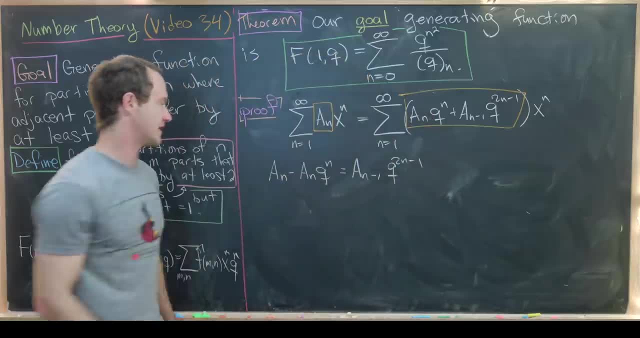 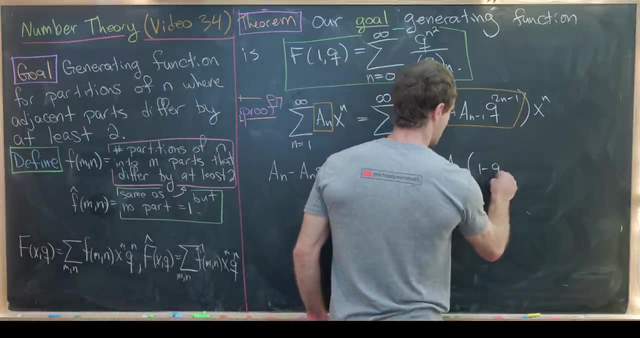 q to the two n minus one after moving this thing over here. Next we can factor an, a sub n, out of the left-hand side. That'll leave us with a sub n. one minus q to the n is equal to a n minus one. 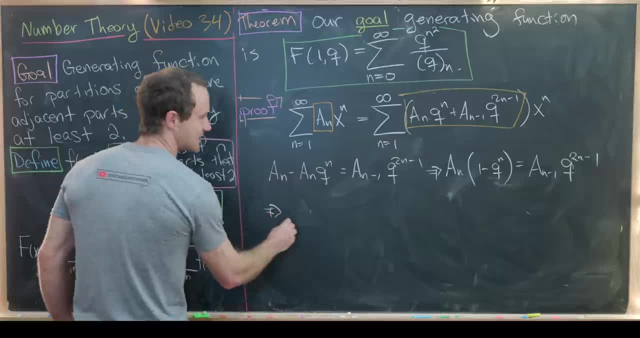 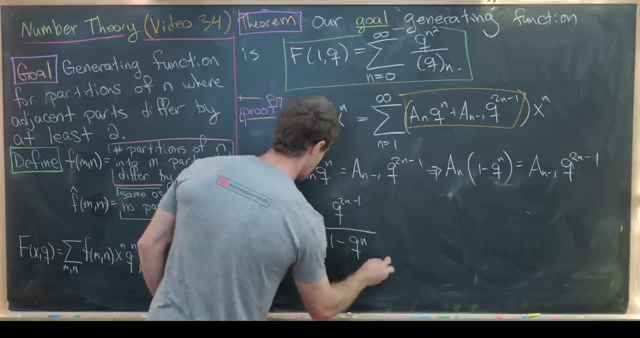 q to the two n minus one. That tells us that a n is equal to a n minus one. q to the two n minus one. q to the two n minus one over one minus q to the n times a n minus one. And now we can just: 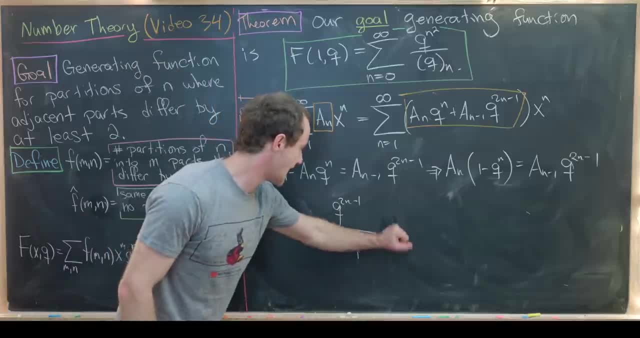 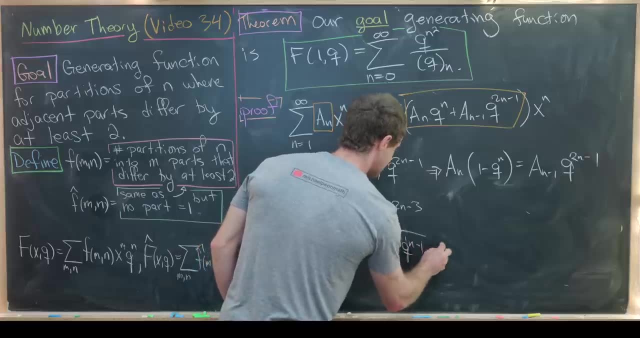 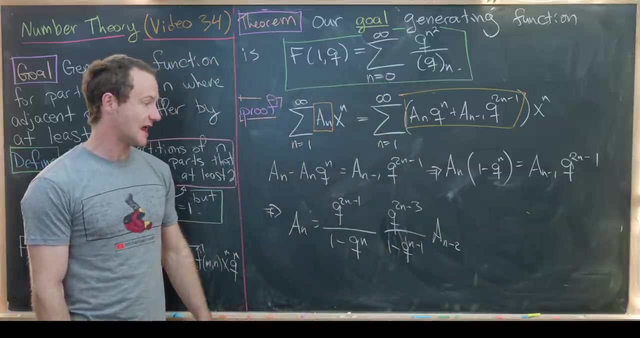 iterate this recursion, So we can replace a n minus one with q to the two n minus three over one minus q to the n minus one, and then we'll have a sub n minus two, And then, likewise, we can replace a n minus two with another term. 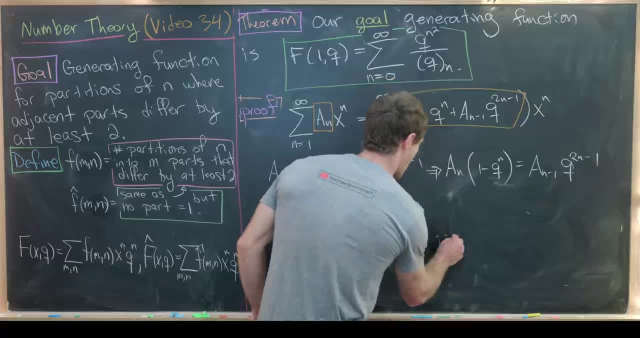 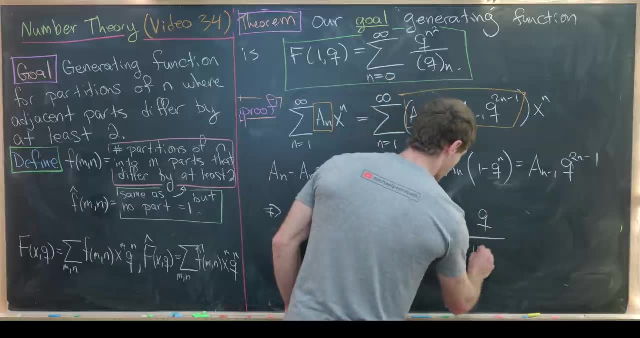 times a, n minus three, And we can do that all the way down until we get a zero, which is one, And then we'll have q to the one, over one minus q, like that. But now, let's see, We can multiply. 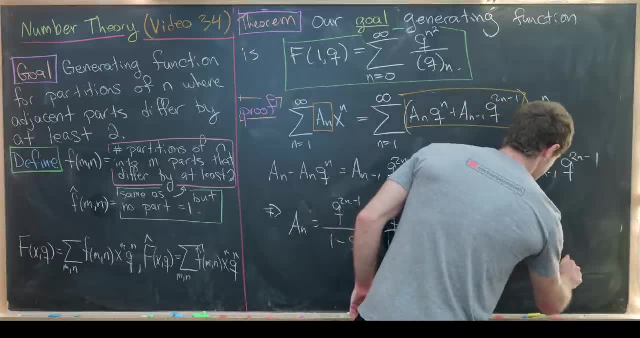 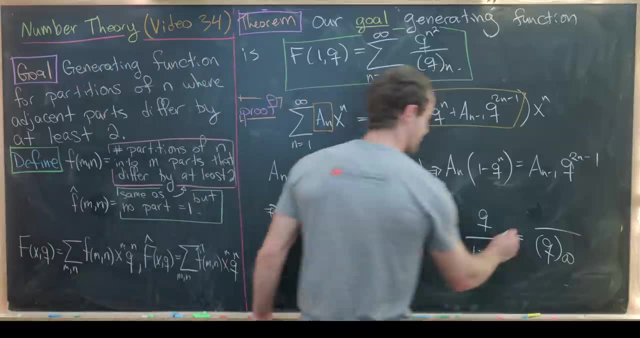 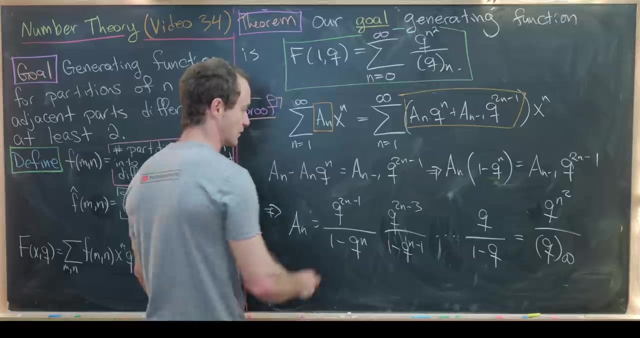 that together. Notice, if we multiply the denominator together, we get exactly that cube-hawck-hammer symbol which is up here. Then, if we multiply that numerator together, I claim that we get q to the n squared. You might say: well, why is that? Well, by exponent rules, what we have up here in the 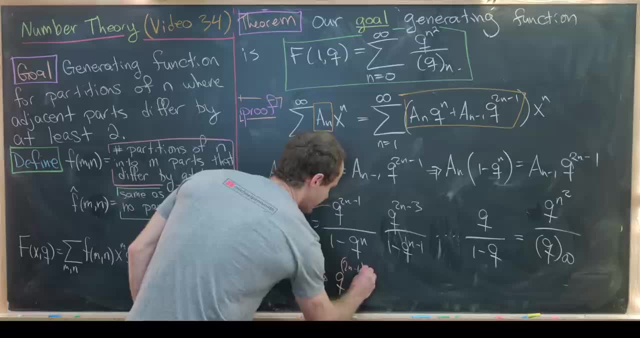 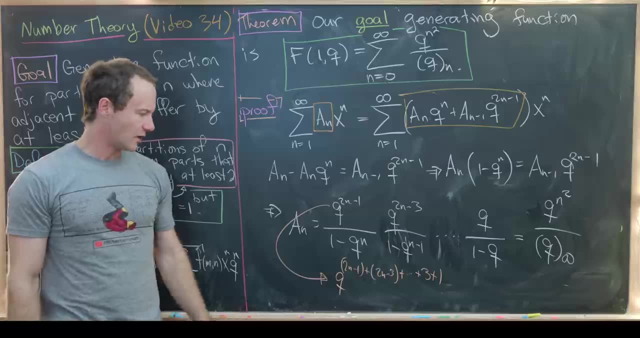 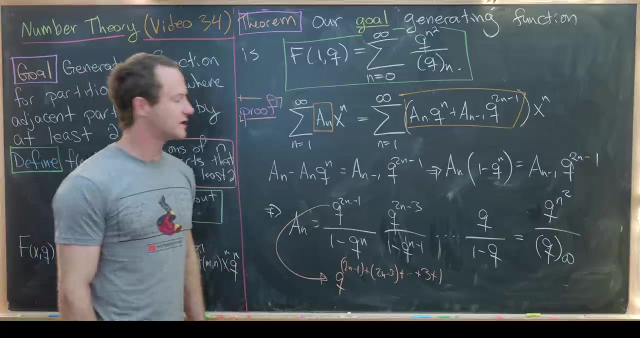 numerator is q to the two, n minus one plus two, n minus three plus all the way down to plus three plus one. But it's well known that if you add all of these odd numbers like this you get n squared. But now let's notice that we're actually done If we take this expression. 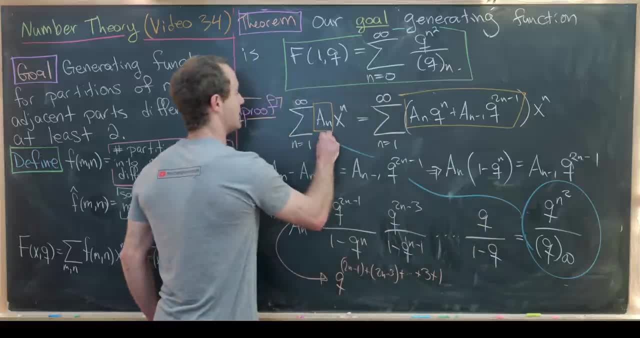 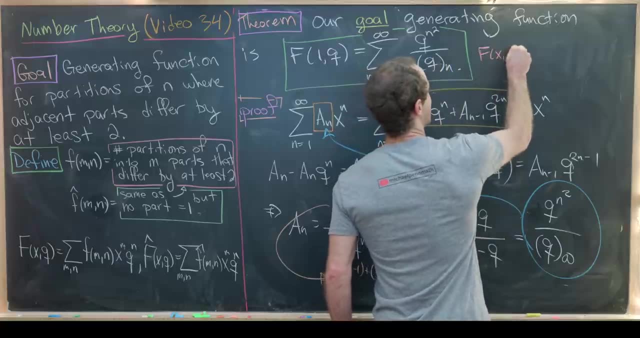 for a sub n and put it back on the numerator, we get a n squared, And then we can multiply that over the denominator, So we get q to the n squared, And then we have actually derived something a little bit stronger than this, And that is that fxq is equal to our sum of. 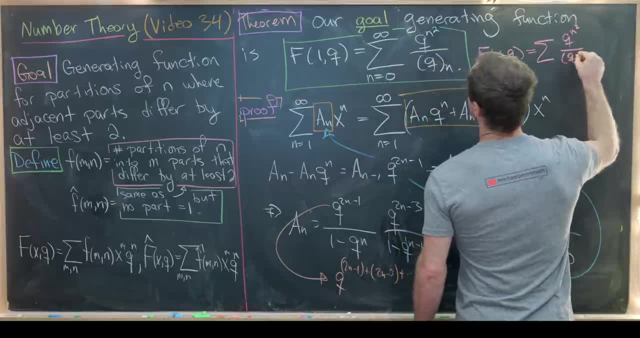 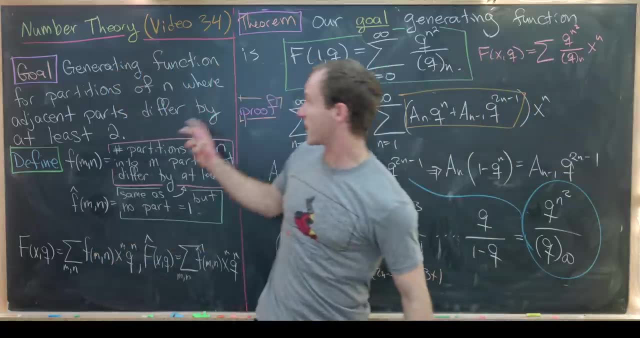 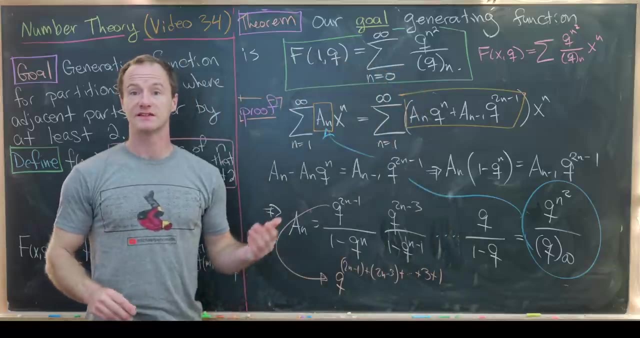 qn squared over qn, x to the n, But then replacing x with one gives us this, which is the generating function for partitions of n, where all of the adjacent parts differ by at least two, And that's a good place to stop.